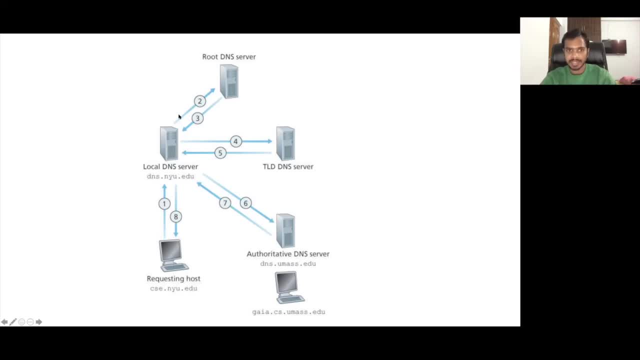 is that in the last video I told you like there will be some query from local DNS server. it is this arrow number two. So there is some query going on from local DNS server to root. Similarly, a reply is there from root DNS server to local. that is arrow number three. So what? 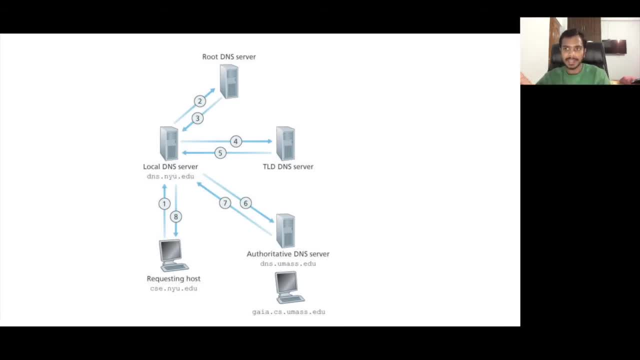 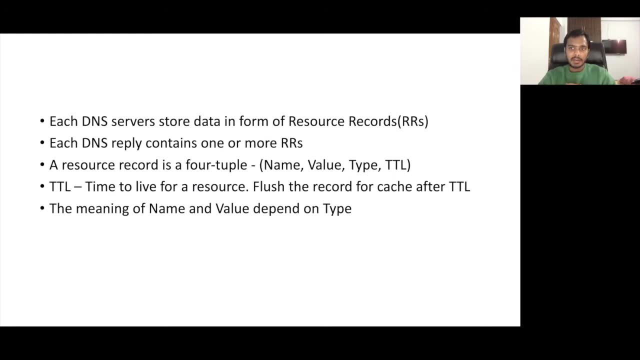 is the actual format of the query and the reply here Similar for others also. that's what I am going to look into, this video. So now coming back to like DNS message format. So understanding resources: We call it very important, So let's look into what this is. So each DNS servers store data. 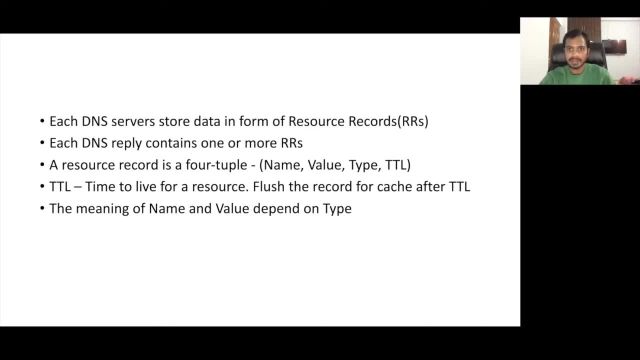 in form of resource reports or results in the sort form values. So there are many types of DNS servers. So you have local DNS server, you have root DNS server, you have tld DNS servers, you have alternative DNS servers. Now, all of this DNS servers store some data and they store that data in the form of resource. 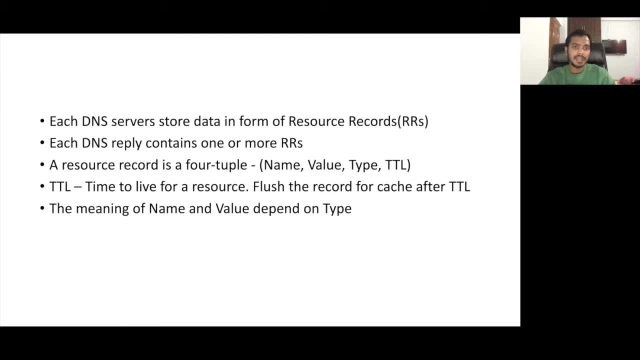 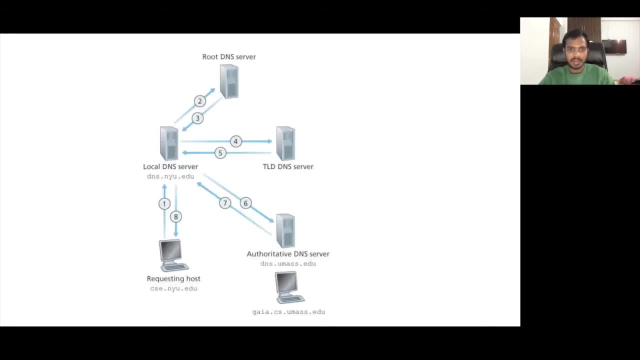 record and we will see later that what exactly they are storing that. Now each DNS reply one or more of more of this uh resource record. so you are seeing here like a lot of replies are there? like arrow number three is a reply, arrow number five is a reply. arrow number seven is a. 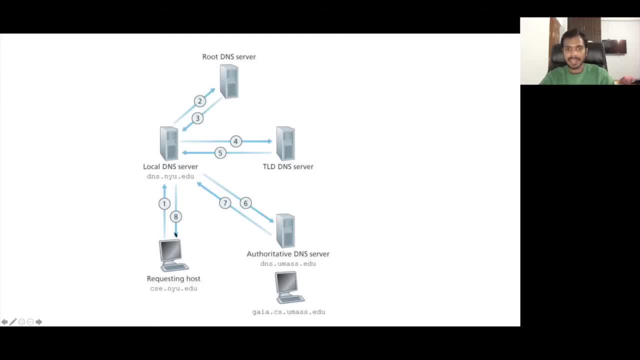 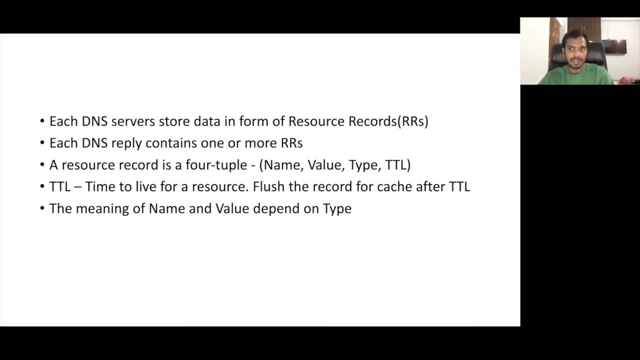 reply. so all of these replies, what they contain, then also, arrow number eight is also a reply. so what the- although all of this reply contains, is they contains, like one or more rrs. either there will be one resource record in that uh reply, or more than one also. we will see in some examples. 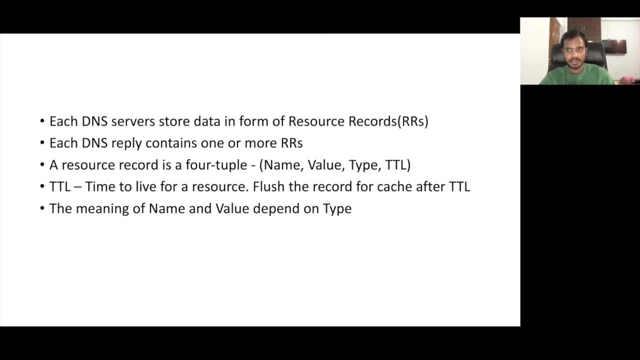 so next question is: what is the resource record? so of course it's a way of storing data, basically right, resource records is basically a way of ensuring data. so you have four tuples here, like you have name, you have value, you have type and you have ttl. so first we will look at the ttl field. 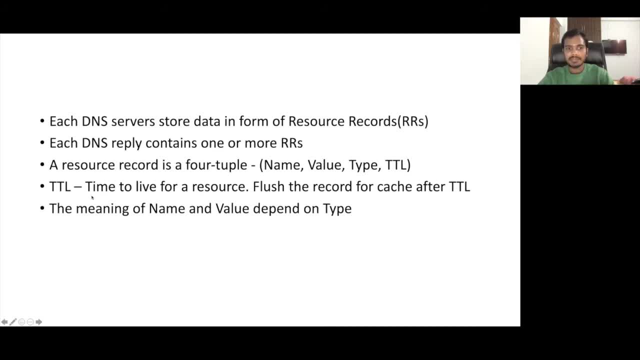 here. that is the fourth field in the resource record, and ttl stands for time to leave. so what is the time to leave for a resource? now, if you remember my last, in my last video i told you that every dns server will also cache the reply. so if you see here, 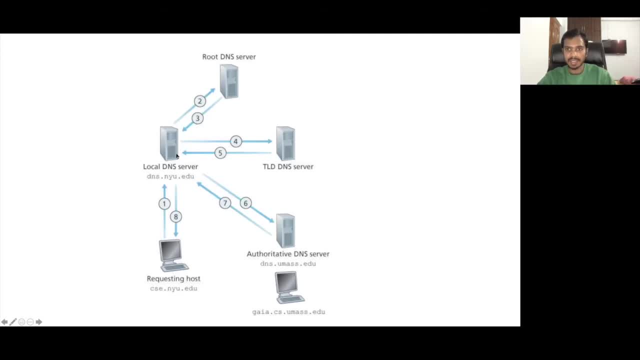 like you have row dns server, so before giving this reply 3 to local dns server, it will also cache this reply in the main memory. similarly, tld will also do the same before sending this. this is the fifth, fifth arrow, this, what is? whatever is there in this reply. it will also. 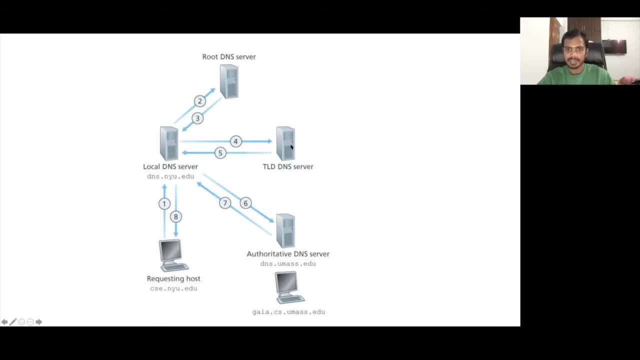 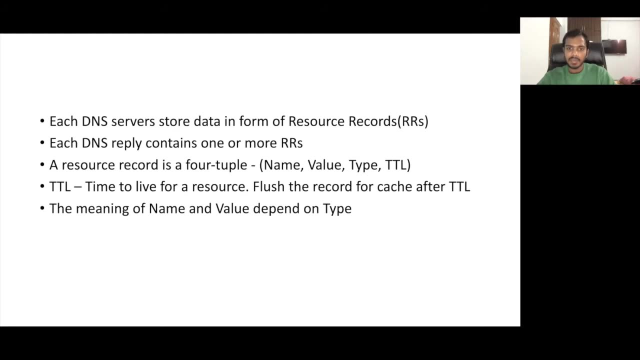 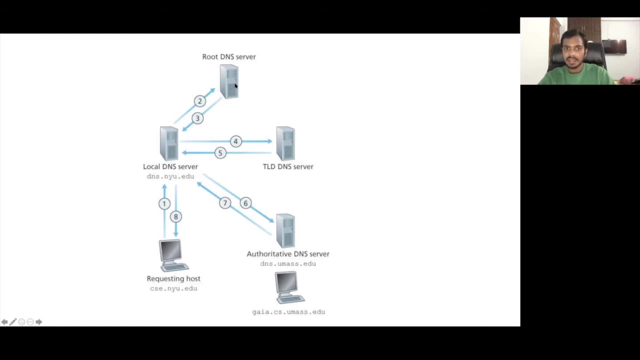 cache that whatever reply is there in the main memory first, similarly for others. also. because of this, what happens? uh, that overall dns system becomes very fast because let's say, uh, of course here, like query number two was there and it has cased that, but if a similar query comes from, 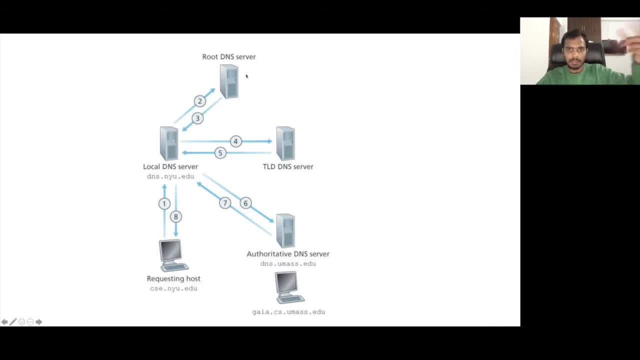 another local dns server. it can reply uh for that query from the main memory itself. it does not have to go to disk and search for that. so it becomes very faster and you can learn more about caching like online, like a lot of videos are there on like how caching uh makes the overall system very fast. 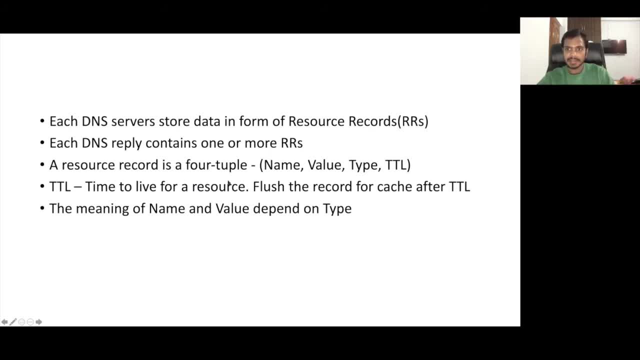 now, after ttl? what will happen after the time to leave expires, then? that whatever entry was saved in the main memory, that will be flushed or removed from that. so that's why it becomes important- because you cannot keep the resource entry forever in the case- because the- i mean the- 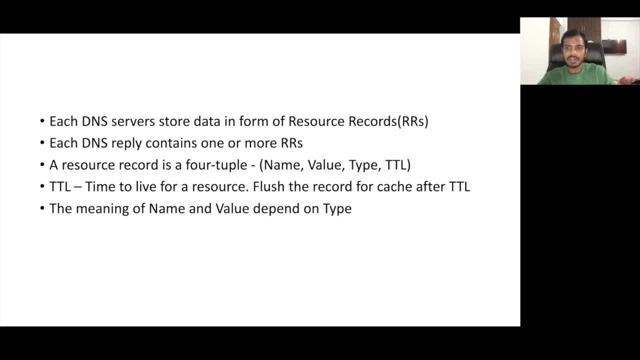 amount of cache memory you have is limited so you have to flush the records after some time. so that's defined by ttn here. so the next thing is: what is name, value and type in resource record? so the meaning of name and value depends on the type. so there can be four types of record. 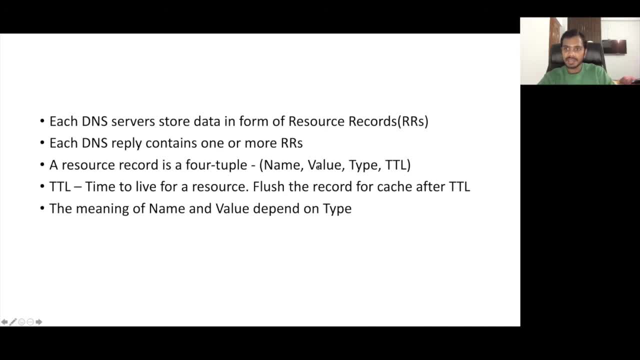 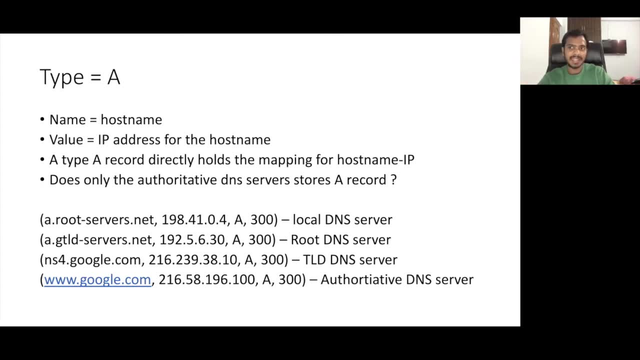 actually we look at each, each of them and the name and value, uh like, will depend on the type actually. so that is very important. so let's look at the first type of records, that is, a record in dns. this is called a recording. dns in this record type equal to a. this is very important. 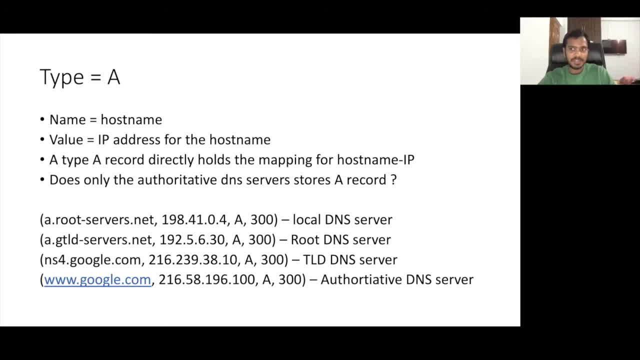 and, as i told you, the name and value will always depend on the type. so when the type is, a name will be hosted and value will be ip address for the hostname. so it's quite easy to understand. in the name field you will have a hostname. it can be any host name: wwwgooglecom, mailgooglecom. 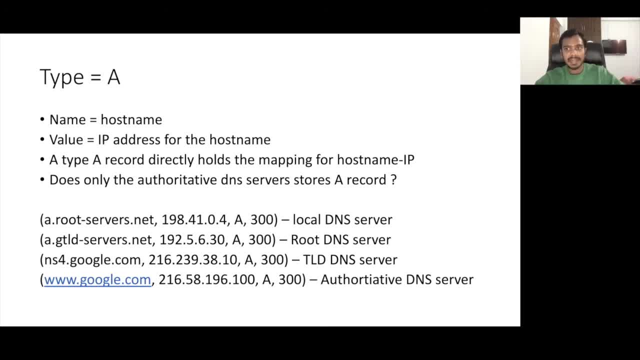 right and what is the value? value will be the: what is the ip address for that host name? so a type a record directly holds the mapping for host name ip. so for one host name, what is the ip address that will be stored in the a record? now you will have the question that, uh, does only the authoritative. 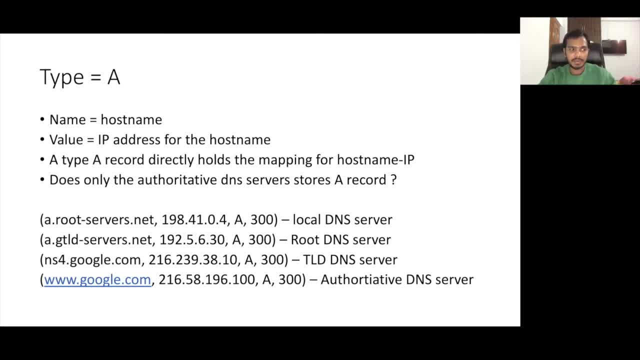 dns stores a record. because if you remember the last video i told that author: authoritative uh dns server was there and authoritative dns server will store the exact mapping of host name to ip address. so of course the question will arise in your mind: that does the only the authoritative. 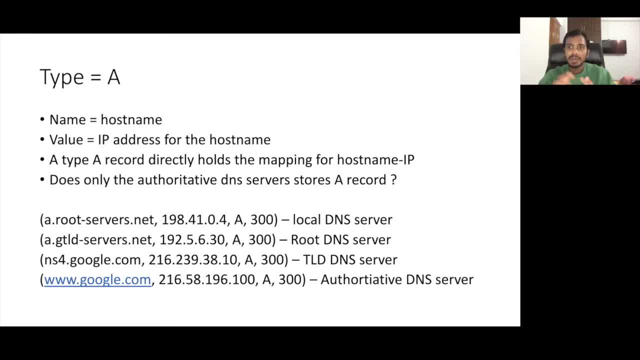 dns server. store this a record? the answer is no, so other dns servers also store a record, but in that case the host name will be different, like i will give you the examples here. see, for example, local dns server. so you see the host name here. this is a dot root serversnet. 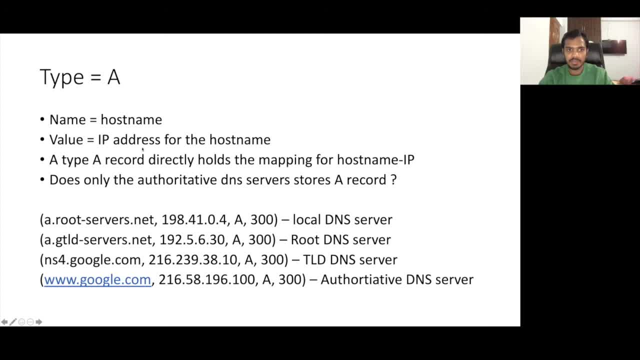 and, of course, as i told you right host name. after the value will be ip address for that host name. this is the value here. so this is basically the ip address of this host name, area dot root and this is a signifies that this is a record, this is a type and 300.ktn here and this: 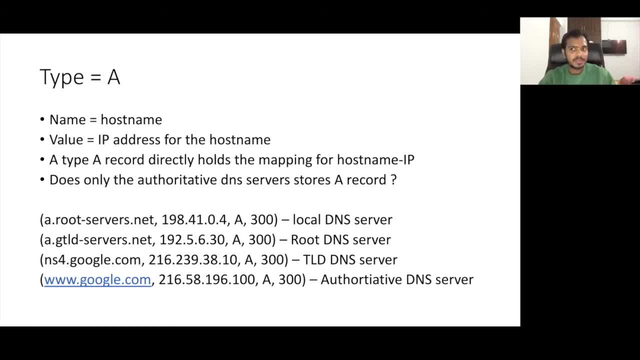 is stored in local dns server. so if you remember what will you just what will? what type of records will be stored in local dns servers? of course the records of, like, the rook dns servers will be 있습니다. so what are the, uh, different root dns servers? so if you see, this is one. 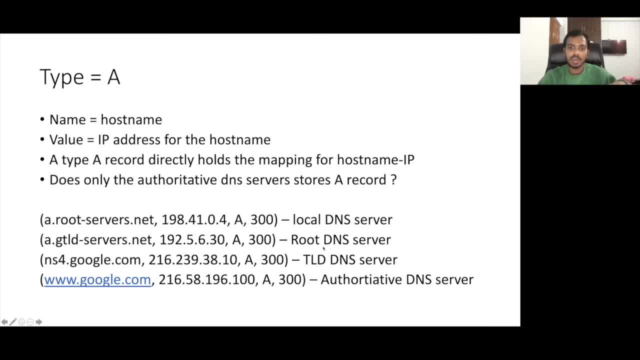 of the root dns servers and that is stored in the local dns server. now if you go to- uh, this is a record- if you go to root dns server now, remember what will, what will be stored- stored in root dns servers. of course you know that the tld host names right and ip their ip address. 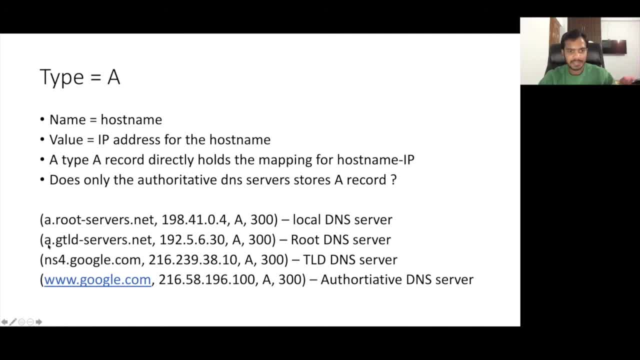 those will be stored in 2dns server. so if you see here this is the one of the host name agltd serversnet and this is one of the host name for dot com tld actually, and the ip address of this host name is 192.5.6.30. this is a record 300 ttl. see in root dns server, local dns server, also a. 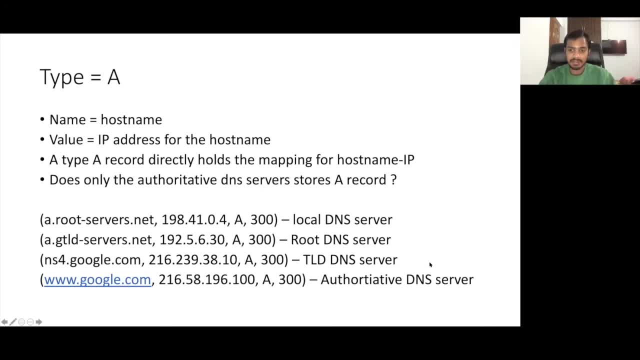 recording is there. even in tld server a record is there, but again, here the host name is one. so of course, if you remember what does tld dns server store, so tld dns server will store information about authoritative dns server, like host name and ip address of alternative dns server. so that's why 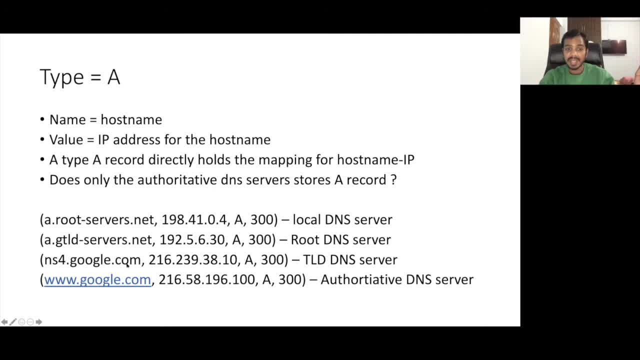 if you see here the host name here is ns4.googlecom and this is one of the authoritative dns server for googlecom, and then you see this is the ip address of this ns4.googlecom. that's what value here. this is a record. there is ttl. 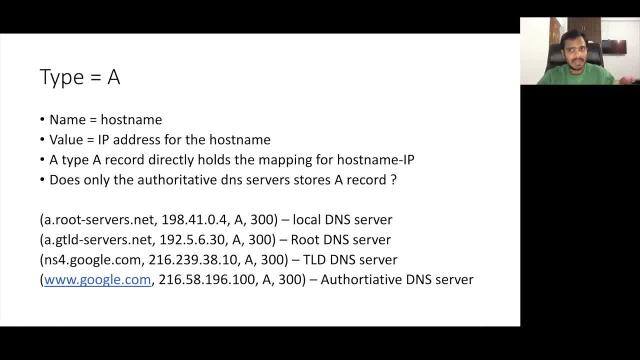 but of course authoritative dns server is the last one and i have already discussed in the last video what is the story of authoritative dns server. so for any website like googlecom or any mail server, mailservercom. so so for that exact ip address is stored. so if you see, 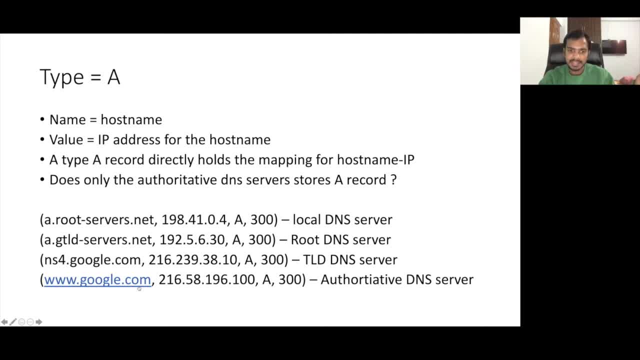 the host name is different. here it's googlecom. this is the ip address of googlecom. this is a record and 300 ttl. so do remember that, like in all of the dns servers, this a record is there, but, again, information storing a record is a bit different. in the 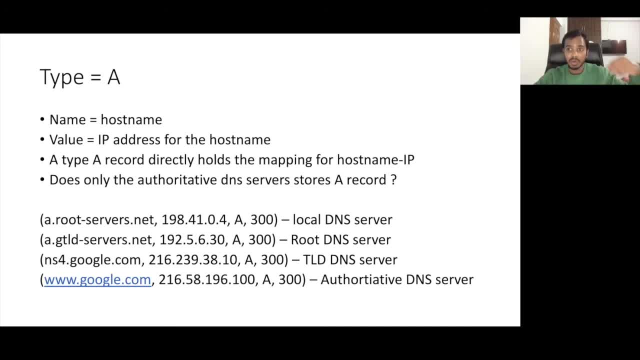 all of this. like in local dns server, the information related to root dns server is stored in root dns server. information related to tld dns server is stored in tld dns server. the information related to authoritative dns server is stored and in the authoritative dns server, like you will have like information about uh websites and all on mail servers and all their. 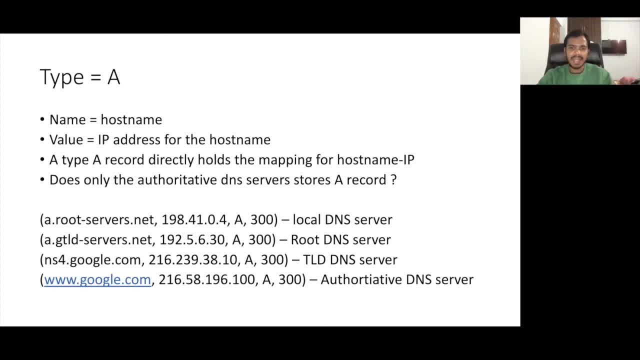 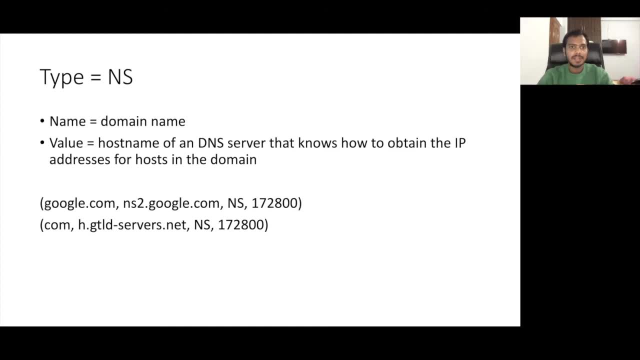 exact ip address will be stored. so do remember this difference. and here i have kept it as like 300 in all of this, but typically this will not be the case. for just this example. i have kept it same. now let's look into a second type of record, that is, anis recording. 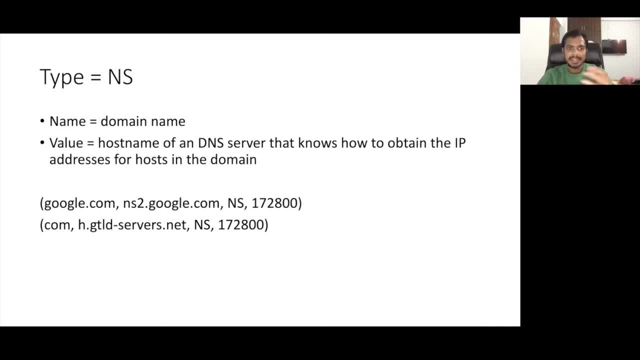 uh dns analysis for name server. now in this case again we have to look into like in this type of records, what is the name and value? this is very important in name. here is domain name, so this can be any domain name, as we see in examples. what is the value? so value is very important here. so 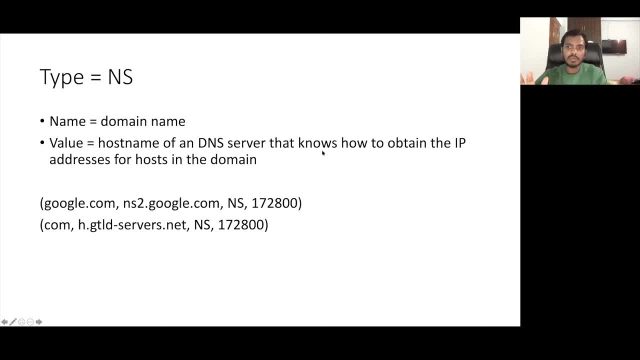 there is a host name of a dns server that knows how to obtain the ip addresses for post in the domain. there will be a host name of a DNS server that can like help you in getting the IP address of host which are there in this domain. So we'll understand better with these examples here. 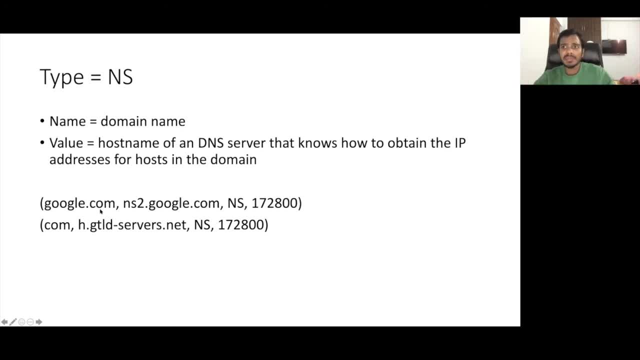 So you have, this is a domain name- googlecom- right, and there will be multiple hosts in googlecom, like mailgooglecom can be there, wwwgooglecom can be there, docsgooglecom can be there, So there can be multiple hosts in this domain. Now, if you want to find IP addresses of different, 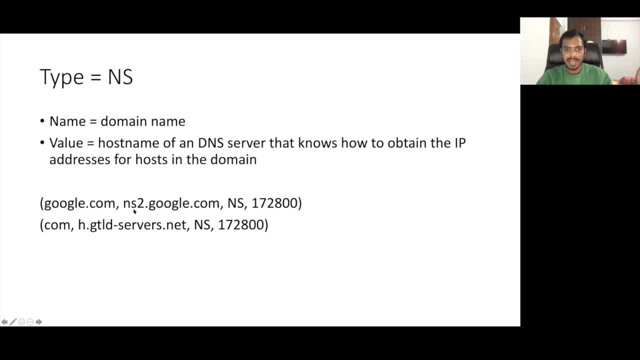 hosts that are there in googlecom, then this at host name, that is ns2.googlecom, can help you in finding IP addresses of those hosts. and this is. you see, this is ns record and this ttl is quite high here. Another example can be like domain, can be maybe com, right, comcom. 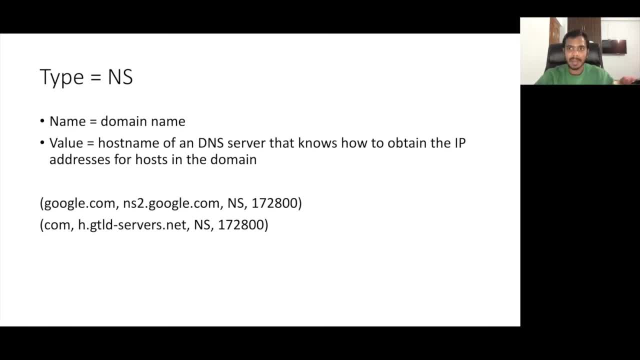 like there can be multiple host names in com, like amazoncom can be there, googlecom can be there and many other others also can be there. Now, if you want to know, like what is the IP addresses of host in? like com, like there are multiple hosts in this, So multiple DNS server. 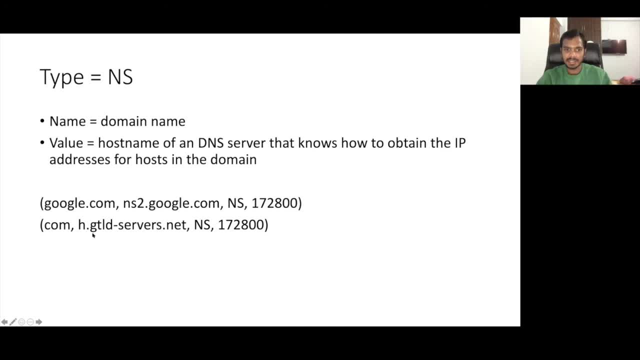 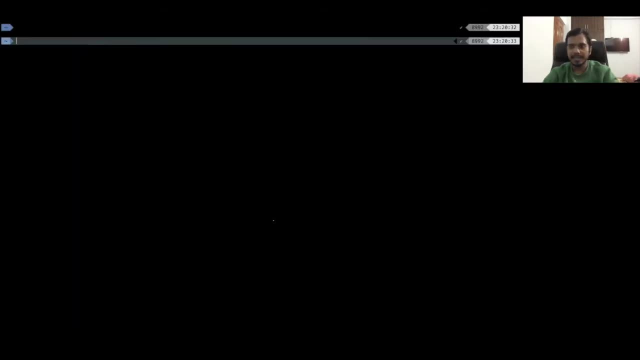 hosts are there If you want to find out. so you can hit this one like hgltd serversnet. So this host name can help you in finding IP addresses of host in this domain, com. and again, this is ns record and it's 172800.. So what we will do now is that we will go to the command line here. 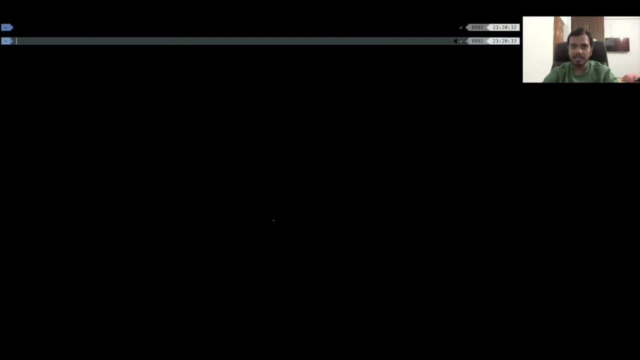 and we will use one of the popular commands, that is, dig command. So this dig command can be used to shoot DNS and also it can be used to like query any of the DNS servers. that also we can do with the help of big command. So see, I will give you examples of like what exactly is stored in all of 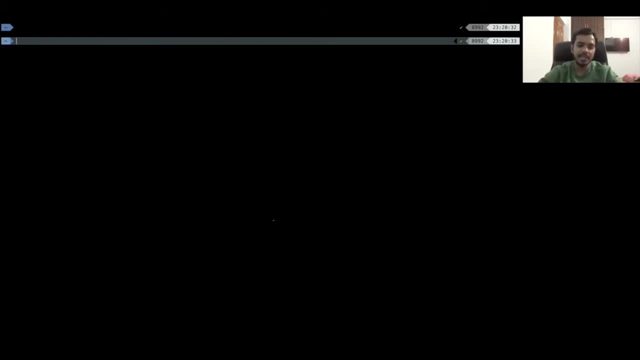 the DNS servers. right, what is a record, ns record? we will see with the help of this commanding command. So let's run this command until, at the rate, we will get one of the root servers, a dot root serversnet. see the syntax of this command. so this is, of course, the dig, is the command here, and 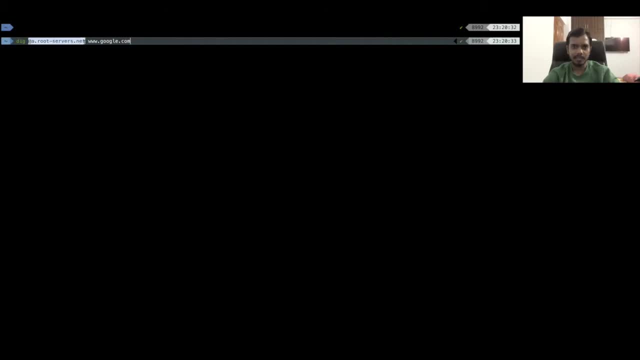 we have at the rate. so basically, this is the DNS server we are hitting. so we want some reply here, like we are asking some questions to this DNS server, and this DNS server here is one of the root DNS server. and then you have this third field, wwwgooglecom. so this can be any domain name or 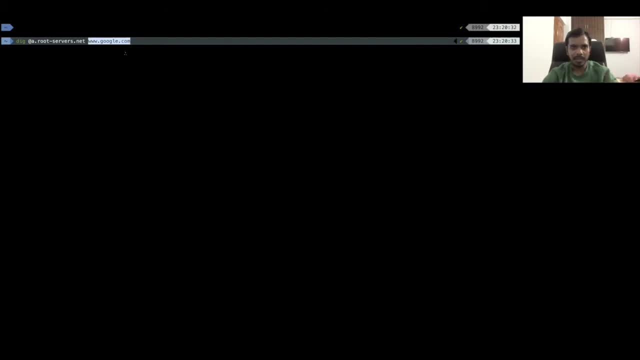 website name for which you want a particular type of record, and here we want a record actually, so you can write a here as the fourth field. that means what we want is, like we are asking to this root DNS server a question, that I want the a record for googlecom, but of course, 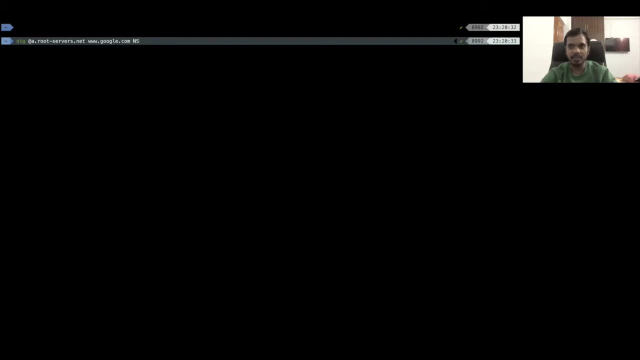 you can also type ns here also, like if you want the ns records for googlecom, you can type ns here also. so by default it will be a record, even if you do not mention in the fourth field, by default it will be a record. so what you will do will press enter and see the output here, which is very, very. 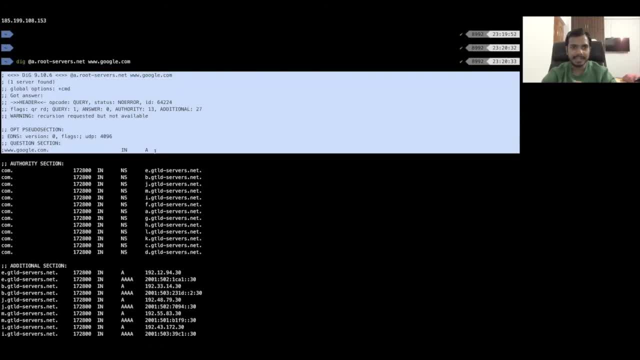 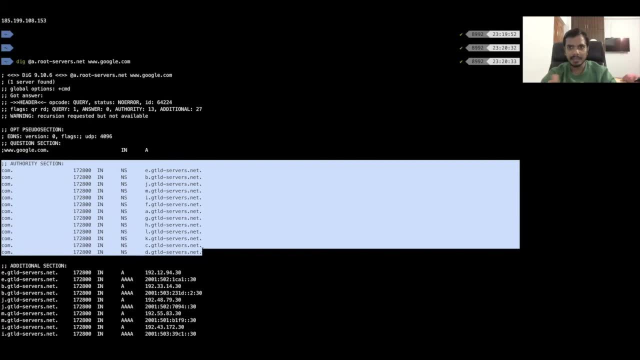 important here. so this first part we have here. I will explain that in later slides, do not worry. but the main important thing is see this authority section. this is very important. so, as you will remember, that the root DNS server will not store the a record for googlecom. 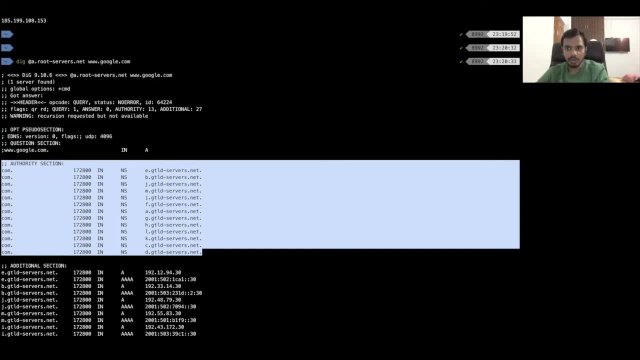 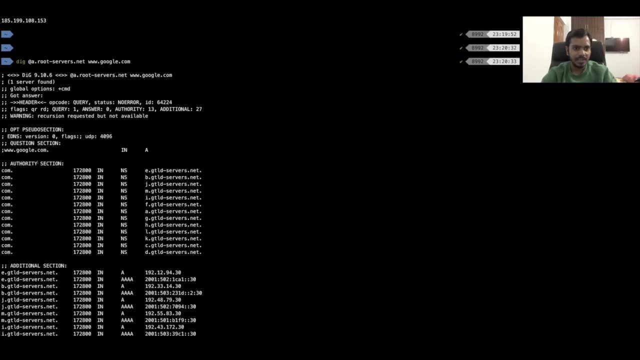 because googlecom, the, a record of googlecom, will be stored in one of the authoritative DNS server right, not in the root DNS server. so that's why, if you see, all of these records in the authority section are ns records, and from here we know what does. ns record stores the value field. 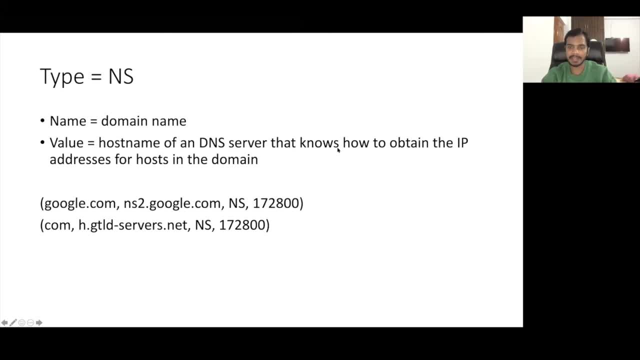 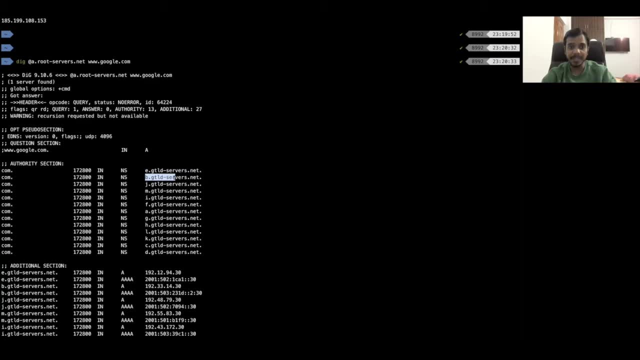 its host name of an DNS server that knows how to obtain the ip address of post in the domain. that means, whatever these host names are here, if you see in the ns records: a dot gtld, b dot gtld. so all the host names that can help you in finding the ip addresses as you set it with the host in. 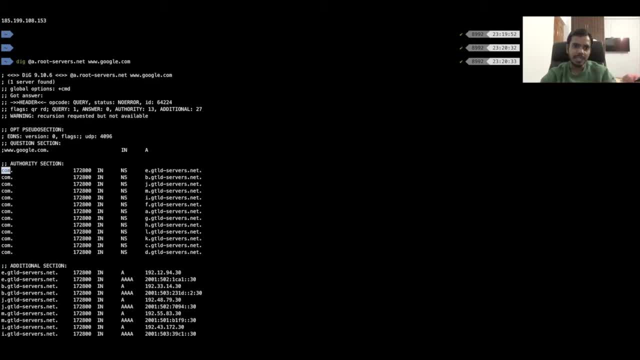 dot com. so, for example, this, this host names- can help you in finding what is the ip address for googlecom, what is the ip address of amazoncom, what is the ip address of, like, yahoocom? so these uh dns servers can help and these, you know, these are the tld dns server and that's what the root. 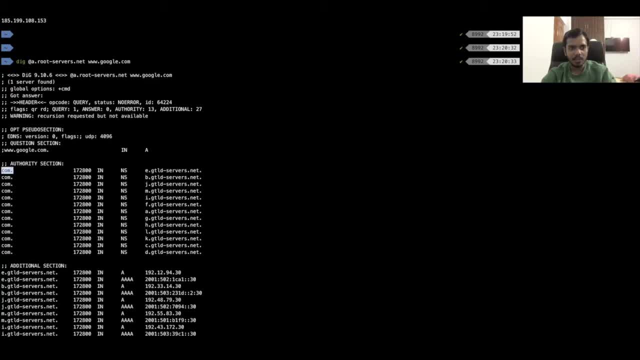 dns server stores and you can see here this is a com dot, so this is basically kind of dot com. this is. this is the first field name field here. this is the ttl here in ns record one, seven, two, eight, zero, zero seconds. this is in. in is for internet. i have not mentioned about this in my 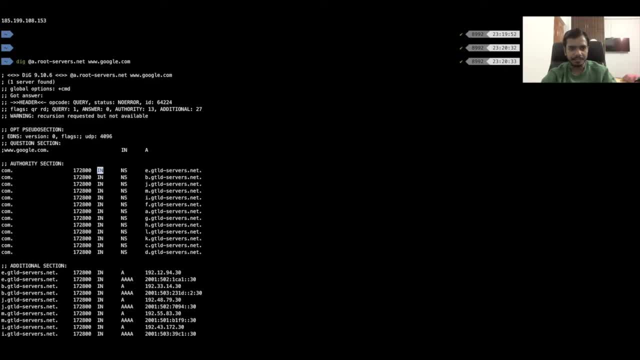 slides, but of course that is an additional field here and you can know, and even google search or more on this, like what actually this field means. then you have ns, so this is ns type of record. this is uh, the last one is the- actually the host name, which can help you in finding the ip addresses for. 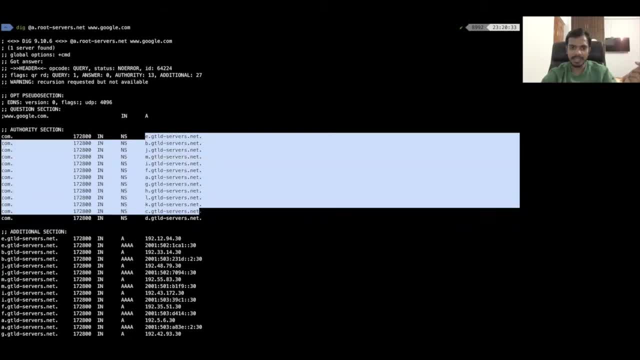 you. there are 13 of them, so this all 13 can help you, so you can hit any one of them and then ask that: uh, tld dns server. okay, tell me what is the ip address of ip address for googlecom? and there is an additional section also here, and do see here that for all of these host names that are here, 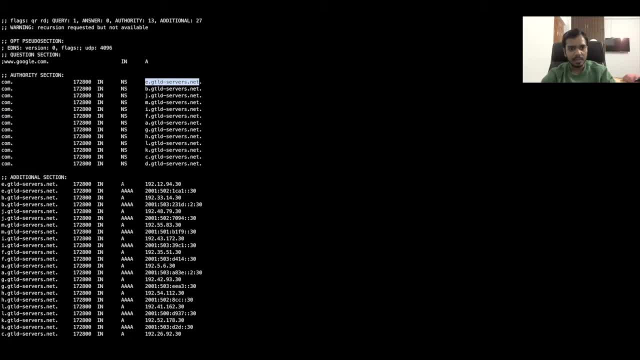 in present here in ns record. there are also a corresponding a record for this and if you see in the a record, what is the ip address for this host name that's present here? so for e, dot, gt, uh, gtld, servers of net, what is the ip address for this? so this is the ip address of this. 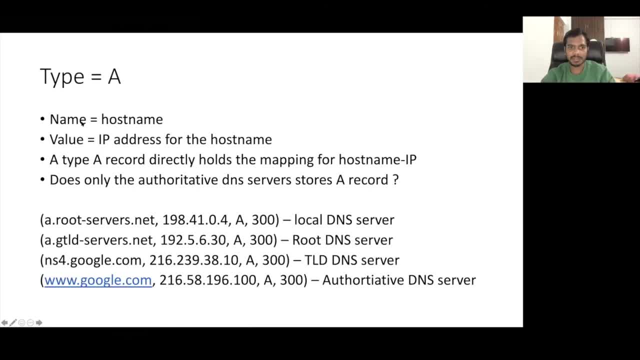 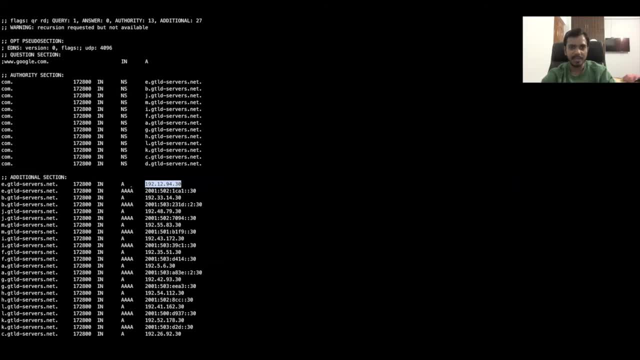 and this is a record. remember, if you go to a record, you know what is stored in a record: host name and ip address for those for that host name and this is very important there. this is the host name and the ip address for hosting a record. and there is like a 4a. 4a is also here. this is another. 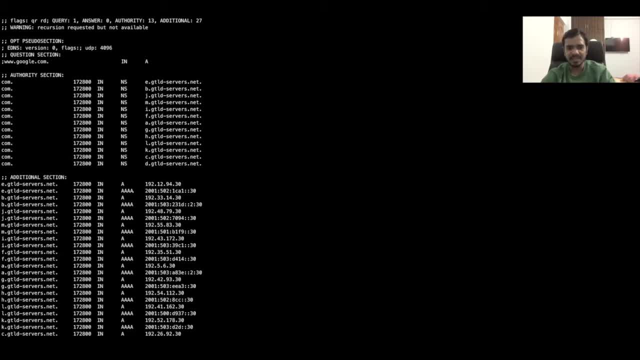 type of record i have not mentioned here, but this is the difference only is that here the ipv6 address is stored for this host name and here in a record, ipv4 address is stored. that's only the difference here. similarly for all the other 13- uh, like tld servers we have, you will see the. 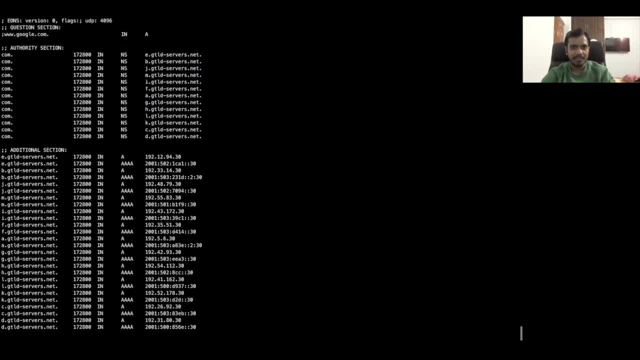 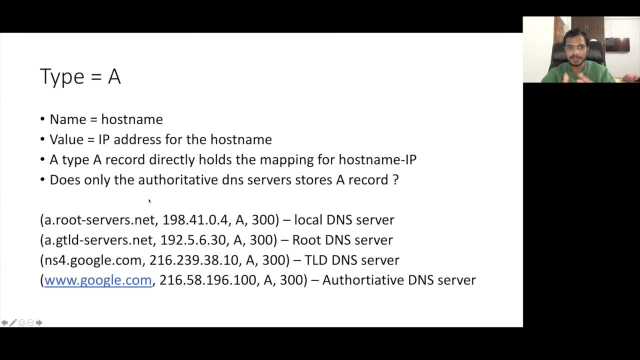 ipv6 and ipv4 address here and you see from which uh dns server we have got this reply. we have got this reply from root dns server and if you remember, and i told you that a records are not only stored in- uh sorry, not only in authoritative dns servers, they're also showing other dns server. 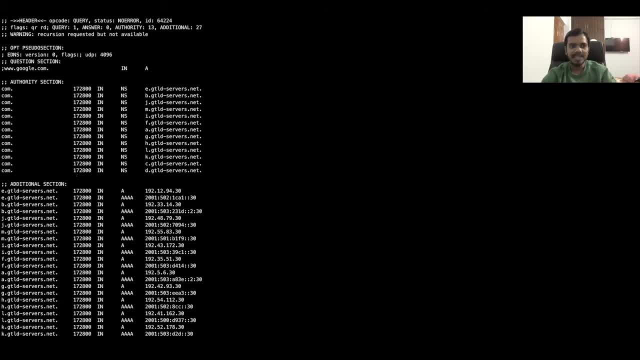 that's what you see in the root dns server. of course root dns servers would have stored this data, right that they only is replying with this data. so in the root dns servers, if you see, of course ns records are there, but other than that a records server is not stored in a record host name. 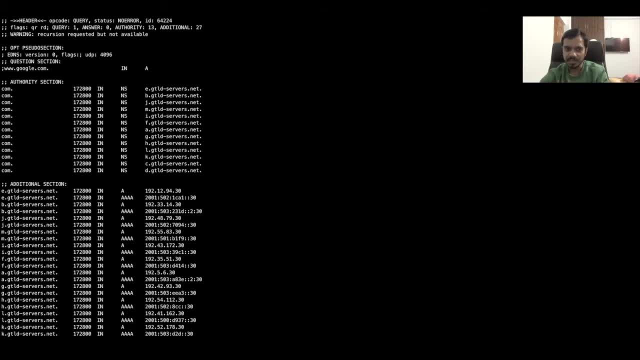 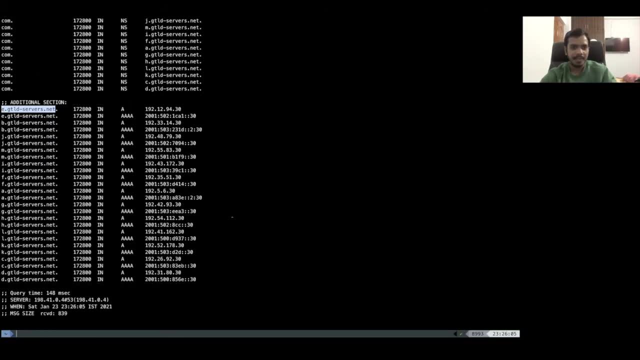 are also there. But do remember that a record- what is the host name is host name is one of the TLD DNS server, So that's important here. That's why these examples makes it more clear And the other a records, if you see here. and okay, one more thing I forgot maybe. 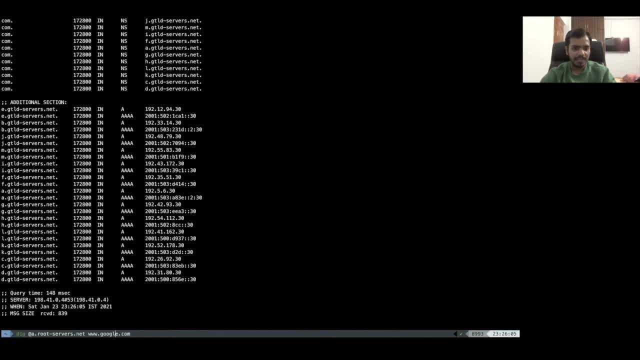 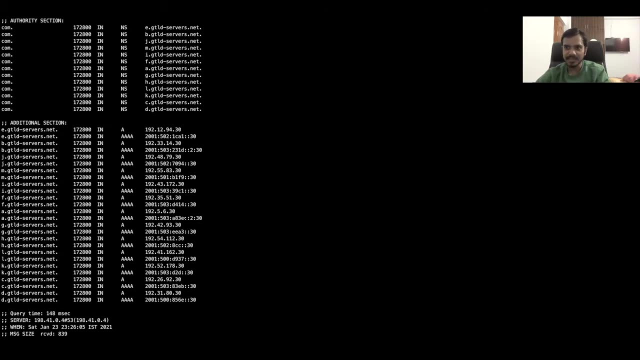 I can show you the chain here. Okay, So after this, what you can do is after this: now we have hit the road in a server, we have not got the exact IP address to googlecom, So let's try to find out that, and this is same as the concept of how DNS works, Like, if you. 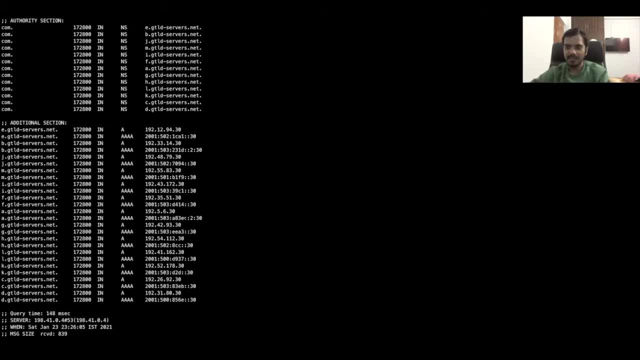 first your local DNS server will hit the route. After that it will hit the TLD. after that you will need the authoritative. So here you do not have a local DNS servers, but we have the dick command to do. do that for us. We will pick up one of the TLD DNS servers. we. 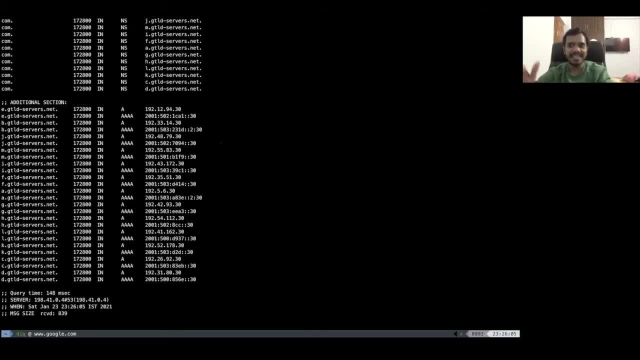 will hit it now. So think about like dick command here as kind of local DNS server that you have there. in the last video we will hit one of the TLD DNS server now. right, Let's hit this, Because we have got reply again here. see the authority section again. 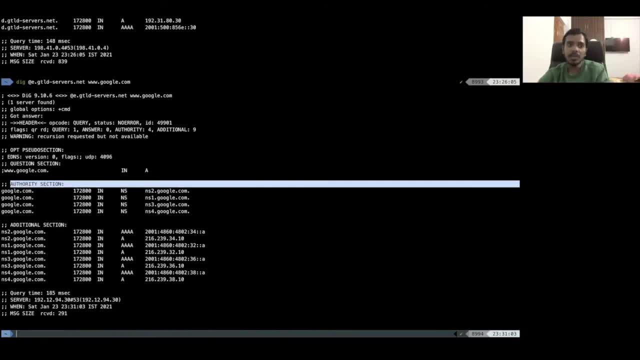 authority section, we have NS records Again. why NS records? Because we know that TLD DNS server does not contain the exact IP address of googlecom. They do not hold the a record for that. So that's why you have the authority section here and NS records, because it is. 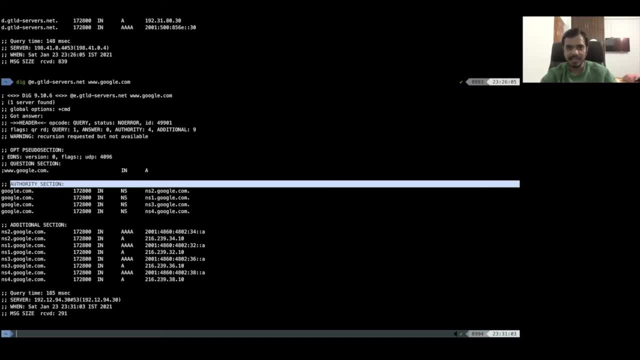 basically, this ejt DNS servers net is telling us that I do not have the exact IP address of googlecom, But these four servers here: NS2, NS1, NS3, NS4, NS5, NS6, NS7, NS8, NS9, NS8,. 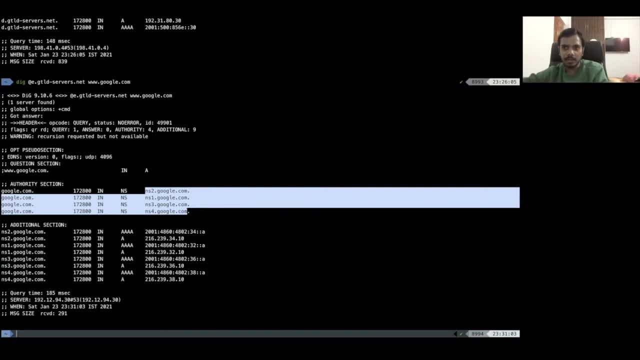 and we got the IP address of 2, 3, 2, 1, NS3,, NS4, googlecom. that can help you in finding out the IP address of googlecom. So that's what is there on the NS record, if you see. 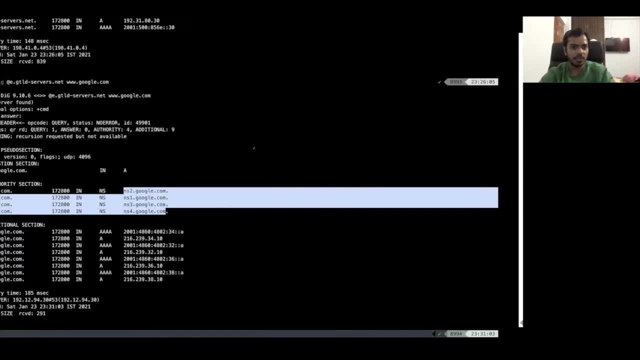 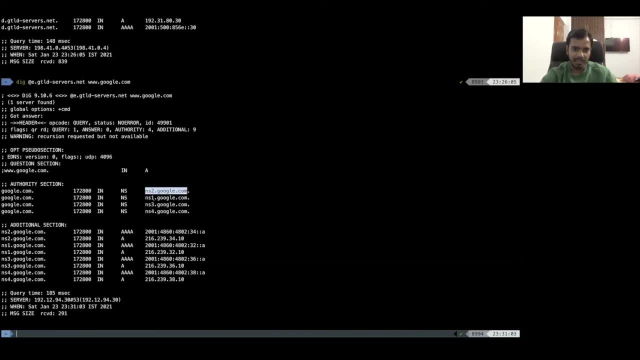 it hosting or DNS server that can help us in finding IP address of hosting this domain of googlecom, Again these similar NS record and if you see additional section for all of these host names like NS2, NS1,, NS3,, NS4, googlecom, What is there IPv4 address and? 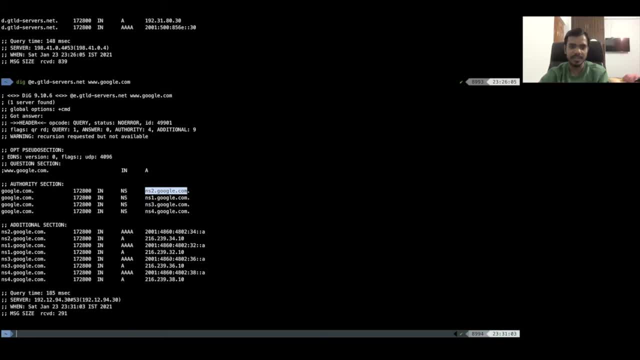 IPv6 address that is told in a record and 4a record. if you see here Now again we have not got the IP address again. So, but we know that these are the actual authoritative DNS servers. So let's, let's hit one of them and S3, maybe you can hit any of them. you should get the. 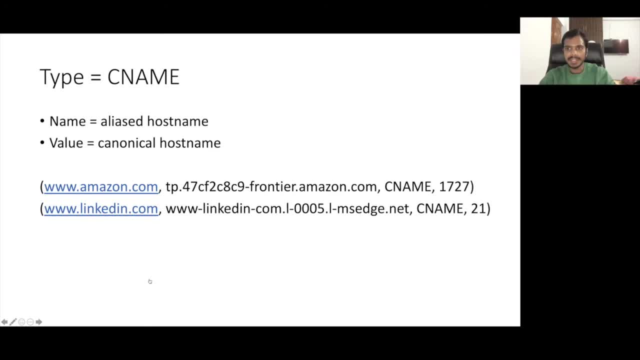 reply. So let's move on to the third category of DNS DNS records, that is, CNAME records. So here, type equal to CNAME. now, in this case, what is name and value? again very important. So name is the alias hostname and value is the canonical hostname. 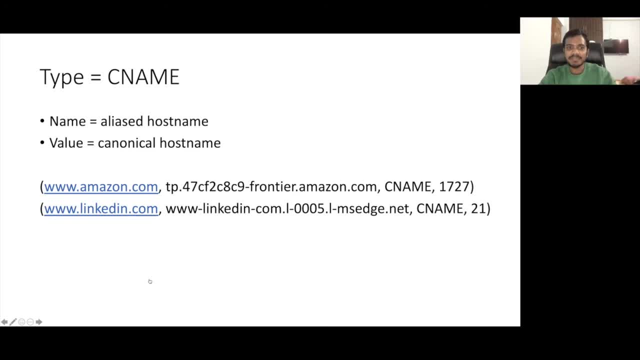 So alias hostname is kind of you can say as a nickname for a actual hostname. So see this example here: the alias hostname is wwwamazoncom and actual hostname, if you see, is tp47frontieramazoncom. so typically canonical hostname will not be very easy to. 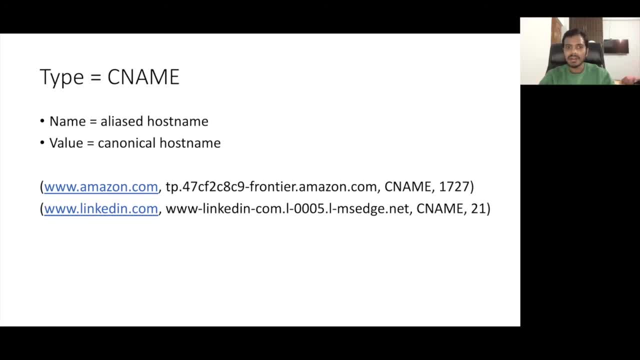 remember and alias hostname will be typically very easy to remember. for example, wwwgooglecom, very easy to remember for us. but if you give some hostname that xyzuswest somethingcom right, very tough to remember those hostnames. so those are canonical hostnames. Again, if you see, this is CNAME and this is 1727. is the TTRN again for linkedincom. this: 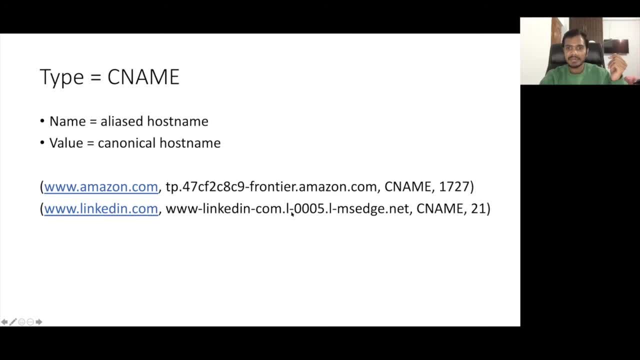 is again like: this is the alias hosting linkedincom and this is the canonical hostname linkedincom. this one and CNAME record and 21. so next question will be like: why are these CNAME records used, right? what is the use of this in the DNS records? so main use of this, I will say, is I will simply: 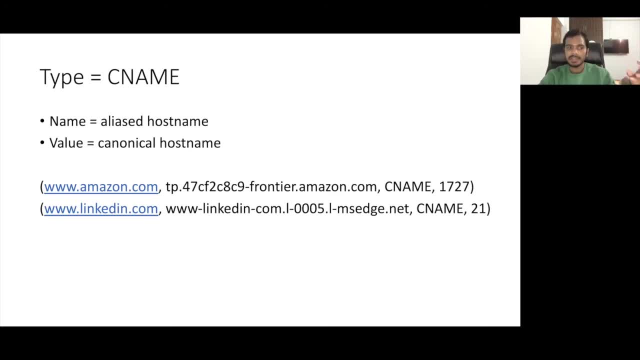 give you an example. so what typically happens is that whenever you are requesting some some thing to amazoncom, so the request will not directly hit the amazon web servers in the sense that see amazon web servers, typically they will be sitting down maybe in US, Singapore or somewhere far away from my place, like I am in India, so they will be sitting very far. 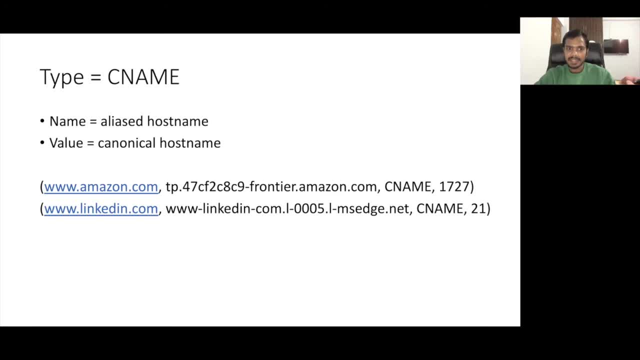 away from me. so what today? like companies like amazoncom, linkedincom, what they will use it. so they will first route my request to some proxy. so maybe it can be a kind of caching proxy, or it can be a proxy for a server or something like that. so they will first. 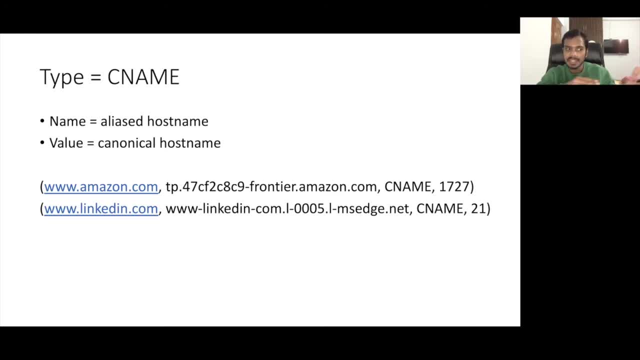 route my request to some proxy, so maybe it can be a kind of caching proxy or it can be kind of gateway kind of thing, right, so basically they will first forward, the browser will first basically forward my request to these proxies, like these caching proxies, and from there 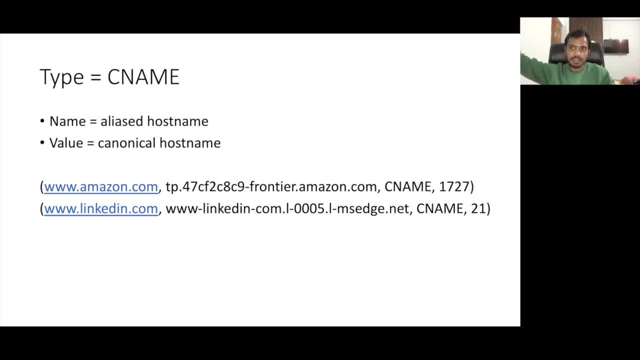 the request will then go to like the servers in the US, actual linkedincom or amazoncom web servers in the US. so that's how most of the like big companies like they do this. now, why they do this is like it's very important because see what there are many used, I mean. 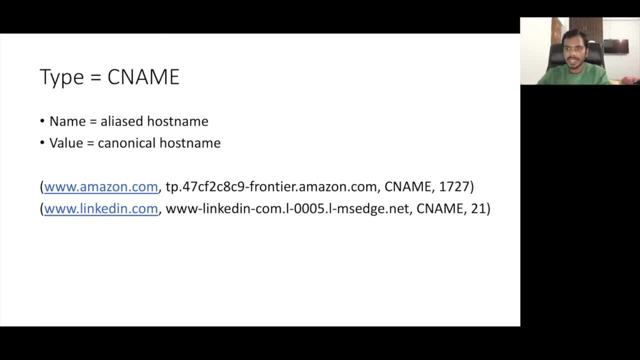 like some people say, like this is the right way to do it. in my case, I mean, like you can use it, like you can find a browser there, and then you go to a server for Instagram and you go to a link to a blog, or you can find a blog and go there and it helps because you 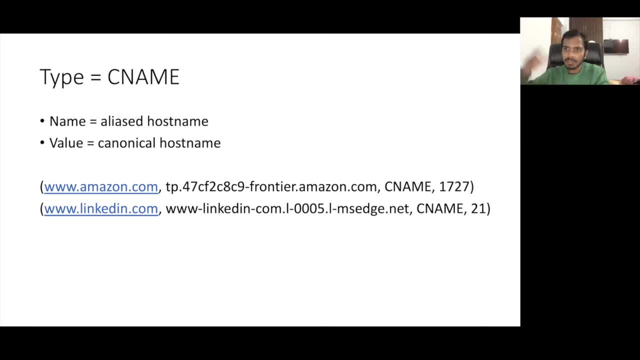 can find something like this and above all and the advantages here is that so this middle caching, proxy or gateway server, so this can of course help in caching. that is, of course, one advantage, and other advantages are also there. like you can the block some IP address, some advantage of this. Now let's see the same on the command line also, like what we 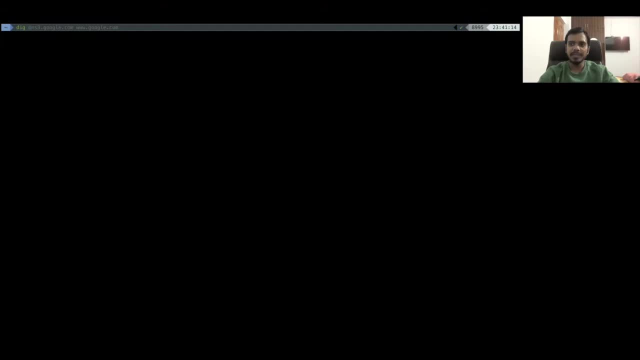 can use is: we can use a dig command, And in this case we are going to hit the local DNS server. So we will not specify the exact DNS server here, But we want, let's say, for amazoncom And we want the CNAME record. So that's what: dig Amazoncom and then CNAME here. Then if 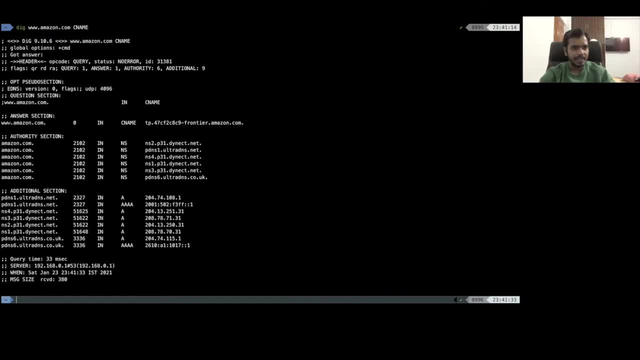 you press enter. so if you see the answer section here, you can see here right there is a record of amazoncom And this is the I mean it is in. there is CNAME, here is zero And if you see this is the CNAME here, TP dot 47. This thing. So of course, whenever 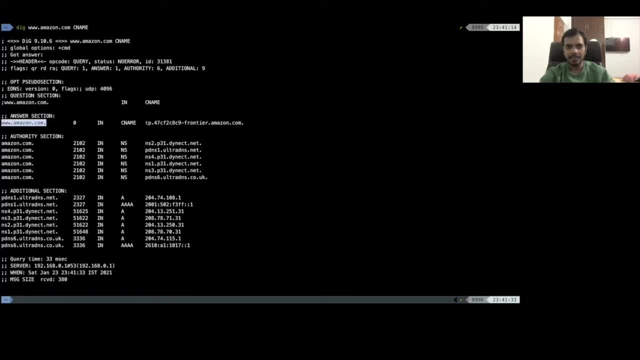 you are hitting amazoncom, the first request will be forwarded to this server. that may be acting as a kind of gateway here in between your client and the actual web servers. And another example also you can see if you want to like. sorry, 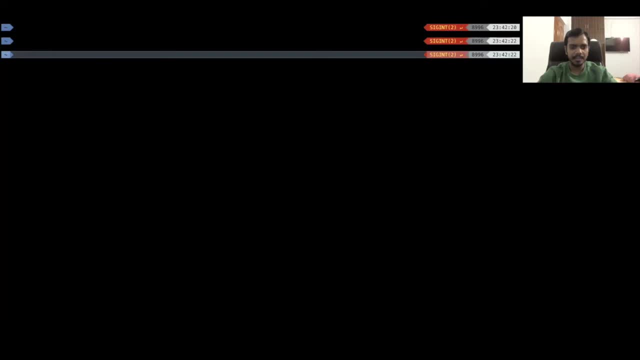 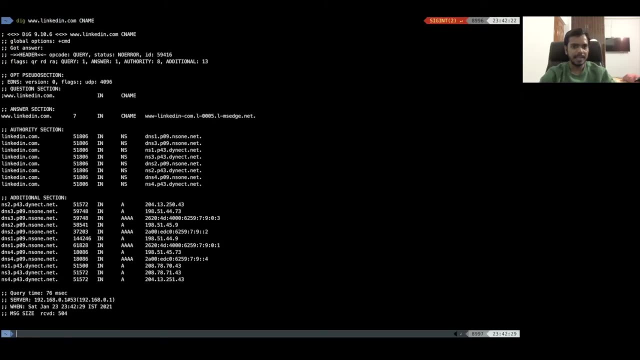 Just let me, let me clear this, And if you take another example, so you can change this to and you can see again the CNAME here right in this, here Again, TTR here is seven. This is the alias hostname, This is the canonical hostname here Another example also I can. 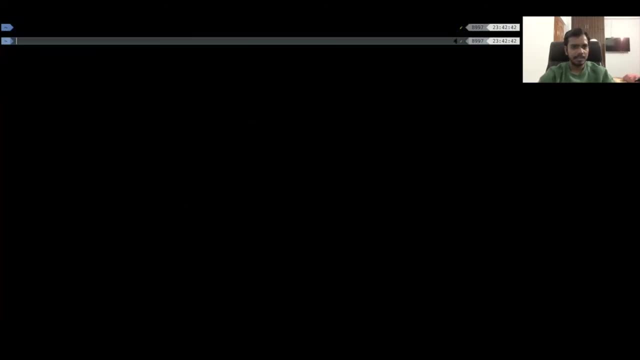 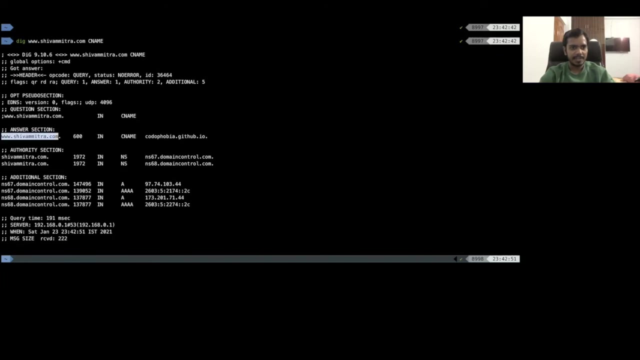 show you. I can show you my website itself. Okay, If you see here, you see in the answer, section alalushivamitracom, a 600 TTR. in again the CNAME and the C. this is codophobiagithubio, So why I'm using this for web, for my website. 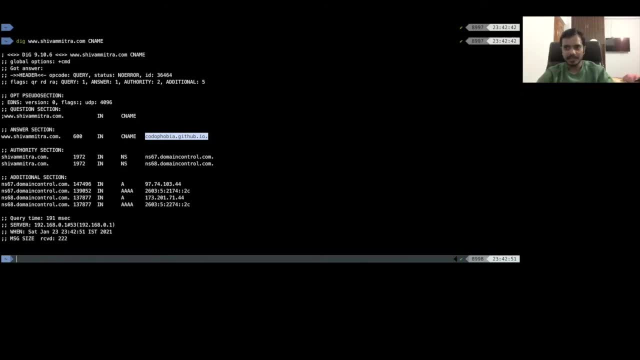 is that. see, my website is hosted on GitHub. Okay, And that's why, by default, GitHub will give you this type of URL, that is, codophobiagithubio. But what I wanted was a better kind of alias hostname for my website, So I went with alushivamitracom And what I have done, so what, of course, I have. 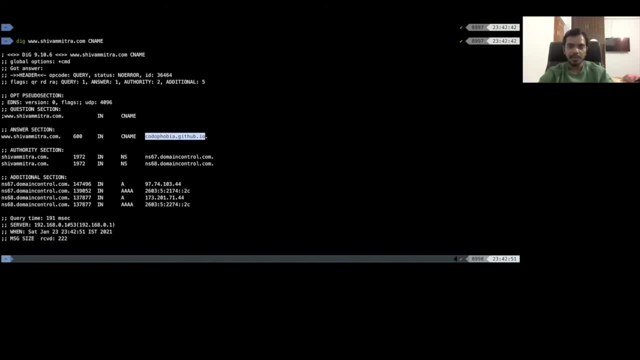 changed the DNS record. So I have bought this domain with the help of GoDaddy, And they also give you the option of changing the CNAME and all. So what I have done is I have pointed this alushivamitracom, basically whenever somebody goes to browser and when they hit. 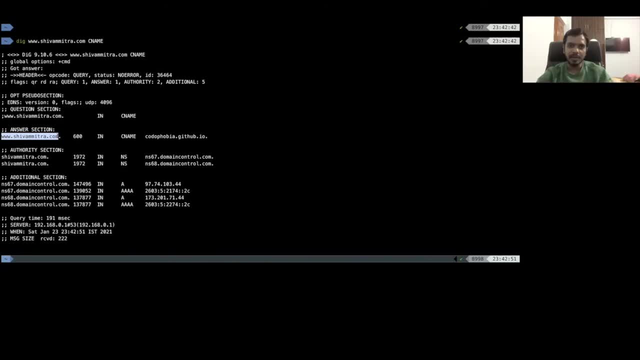 alushivamitracom. the request is forwarded to codophobiagithubio. and that is actual. the GitHub is hosting the website for me. Okay, Okay, and then it will serve the request from this one. it again. this will again. this also, you can resolve. 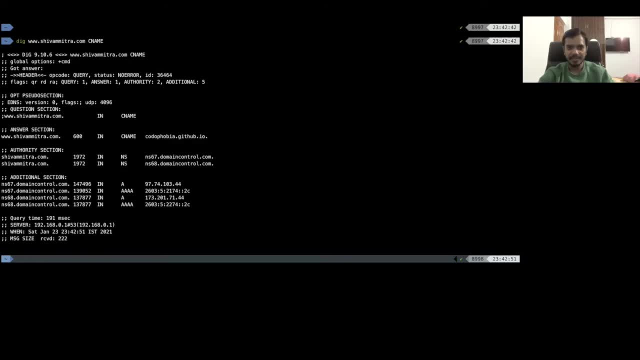 for this. also there will be ip addresses. of course you can find the ip address for this. so we, we only need a host name here. so of course, again, you can use the dig command. just mention this here, okay and okay, just run, you will get the ip address. so if you see in the answer section here like there, 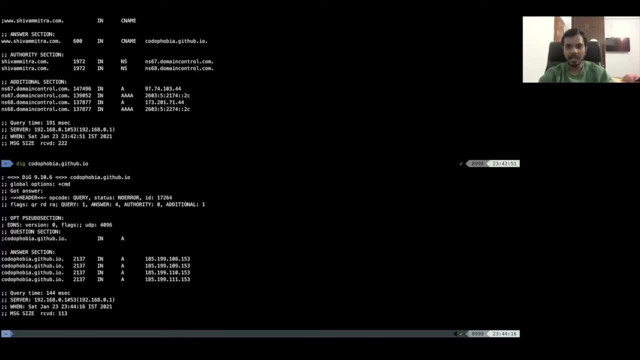 are four a records. so basically for this codophobiagithubio you have four different kind of ip addresses. if you see right this, all four of them are there and all four of them will do the same thing. i mean whenever i make a request, so this request can go to any one of them, any one. 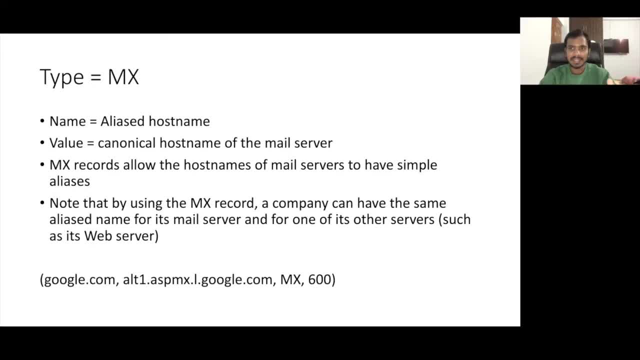 of the ip address and they will serve the request. the next one is type equal to mx and this is also very important because this type of records are used to like a store. i will say the mapping of host name, ip of email server, so we will see what that is. so here again, if you see name equal to, 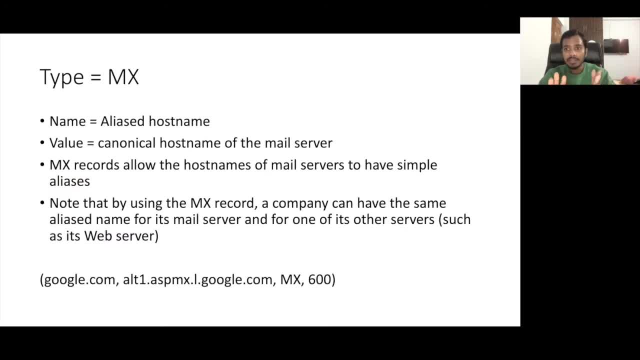 aliased host name, similar to type of cname, but value. look at the value here, like in both the cases, is it has different context. their value equal to canonical host name. again canonical hostname and the same one, but see the next line, canonical hostname of the mail server. now this line differentiates between the mx record and cname record. so in the cname 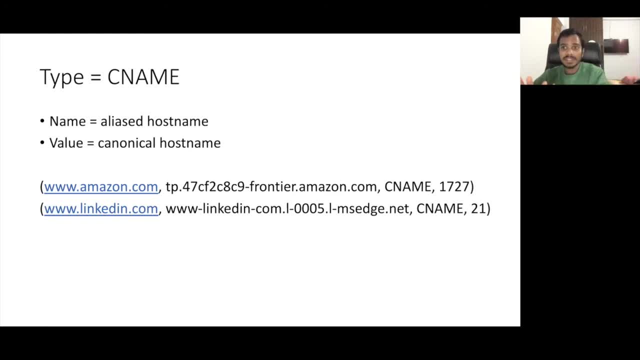 record. there is canonical hostname, but the canonical hostname is not of a mail server. it can be any other server, it can be a web server, it can be ftp server, it can be any other server, but it will never be a mail server in this cname, unlike cname record. 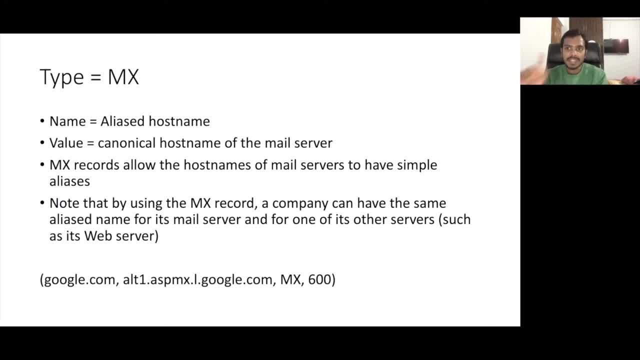 But in case of MX record, the value will always contain canonical hostname of a mail server. Do remember this is very important. You'll see examples also. So MX record allows the hostnames of mail servers to have simple aliases. So, of course, again, mail servers. 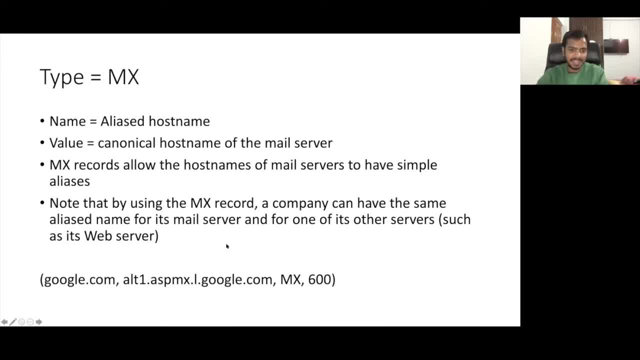 I mean their canonical hostname will be very different, Like- take this example- alt1aspxlgooglecom. So you will not remember. it's very tough to remember this type of canonical hostnames, So we'll provide an alias hostname for this, For example. 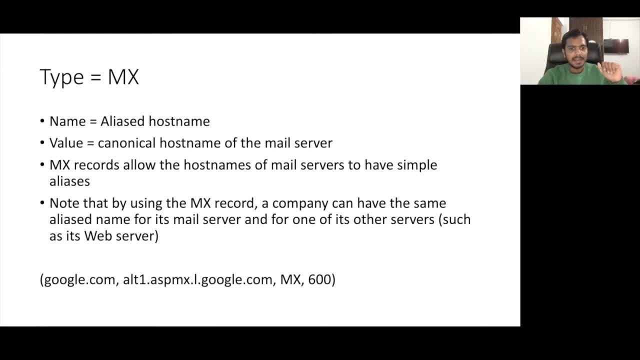 googlecom is the alias hostname here for this. Now, if you see, the third is MX. this is quite important. here CNAME and MX are quite different, So here the record is MX. Do note that by using the MX record a company can have the same alias name for its mail server and for one of its other. 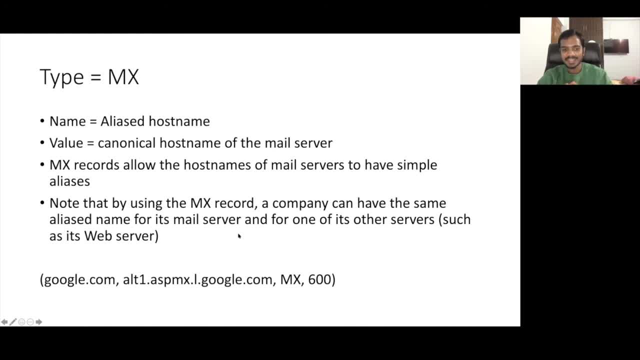 servers, such as its web server. This is very important actually. So using this concept of like MX and MX record, you can have the same alias name for your mail server. So, using this concept of like MX and CNAME record, what you can do is see in this example for googlecom you have 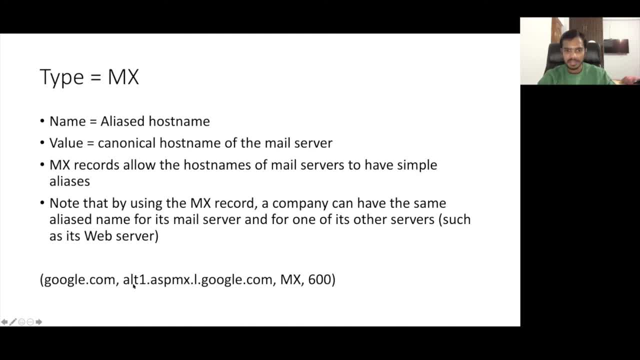 this other canonical hostname And this is MX record. So basically this googlecom in this case is pointing to a mail server. But you can again have another record, similar record. You will again have the first as googlecom, But in the second, like in the value field, you can have. 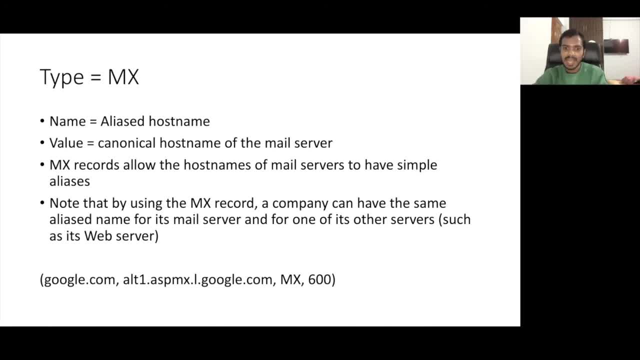 the canonical hostname of a web server or FTV server And in that you can change MX to CNAME here And you can put anything. So basically, you can have the canonical hostname of a web server or FTV server And in that you can change MX to CNAME here And in that you can put anything. 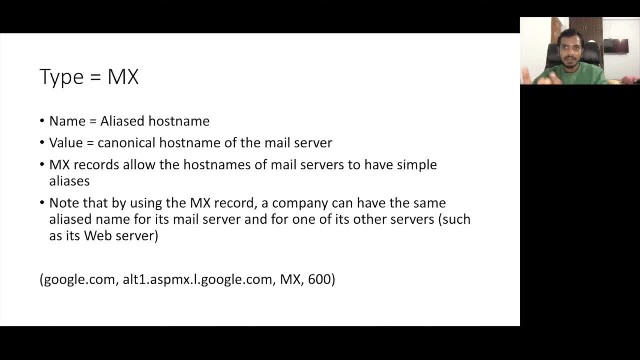 you can put any. I am just giving an example. See what happens: With the help of same alias name, that is, googlecom, you are pointing to two different servers. So, through the help of MX records, you are pointing to one of the male servers of googlecom Through the use of CNAME. 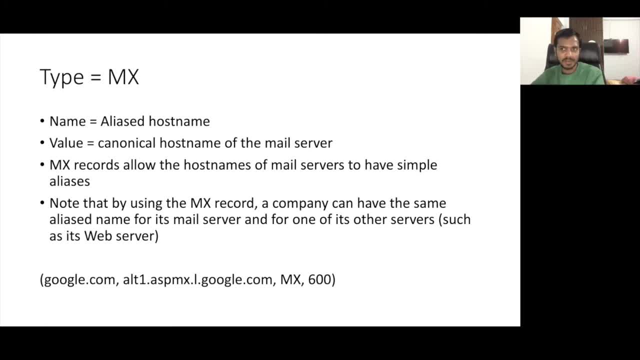 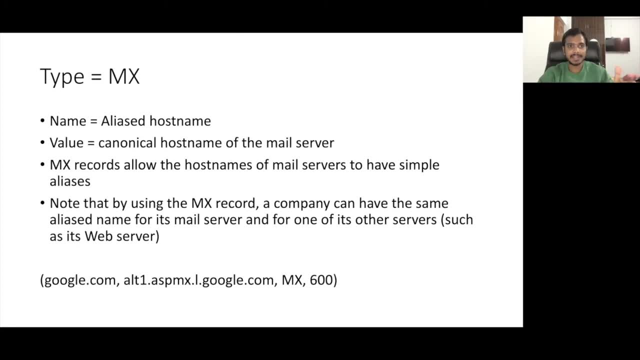 record. you are pointing to one of the wave servers for googlecom. See the magic, With the help of- I mean same alias name- what you can achieve through MX and CNAME record. Now let's see the example for type equal to MX, which is again very important. 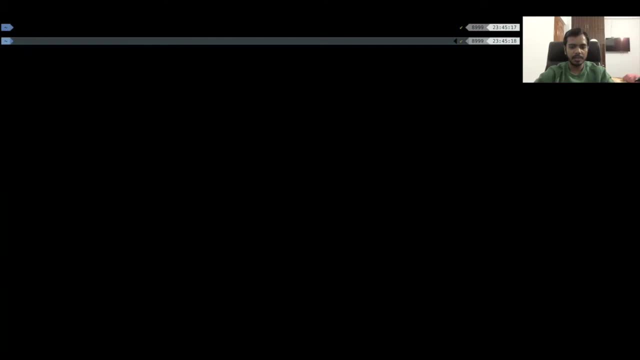 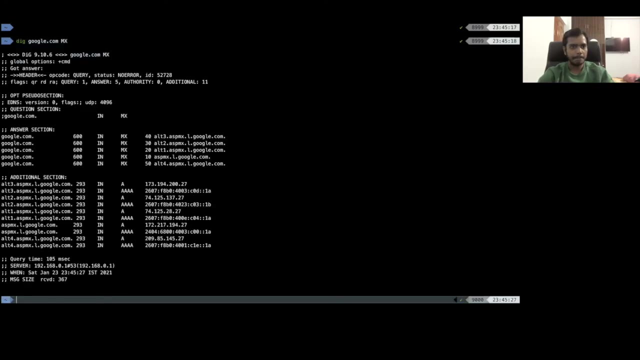 So what we will do is we will take the example of googlecom itself. dig googlecom, and we want the MX record here, So you can see here. so, basically, what does this mean? What does MX record mean? So in one sense, I will also give you the importance of this. 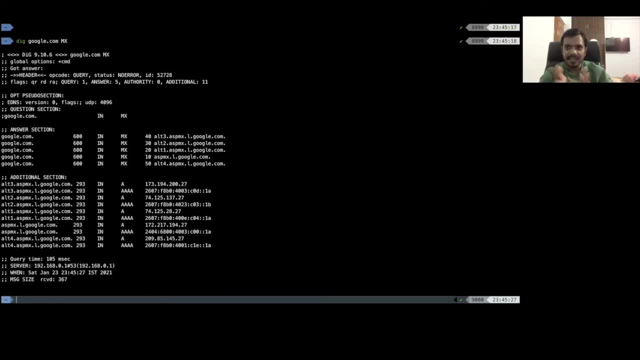 So whenever somebody is sending a mail to x at the rate gmailcom or y at the rate gmailcom right Now, where should this mail be stored? So these mails are typically stored in mail servers. So what you are seeing here is that mail servers like alt3, aspx- lgooglecom. 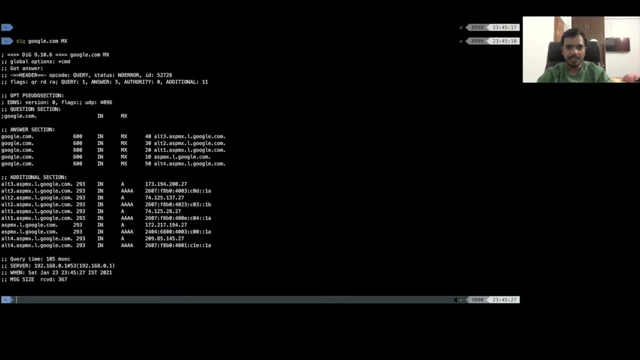 like there are five of them, So these all five. if you see the host names here, so these are basically the host name of the mail servers associated with googlecom. So whenever you send a mail to like, a at the rate googlecom, b at the rate googlecom. 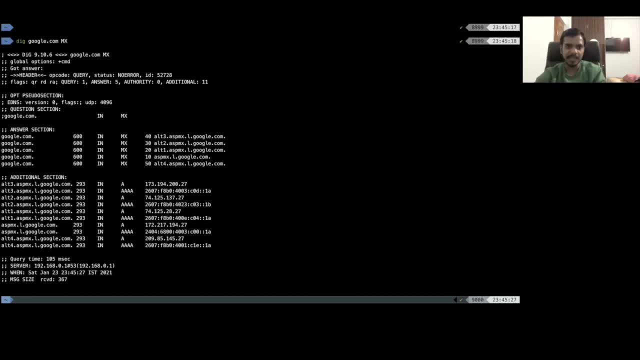 just give some examples. Those mails will first go to these mail servers that are here And you can see this MX record again: b at the rate, googlecom. this is basically your alias host name. ptl600, in is internet. 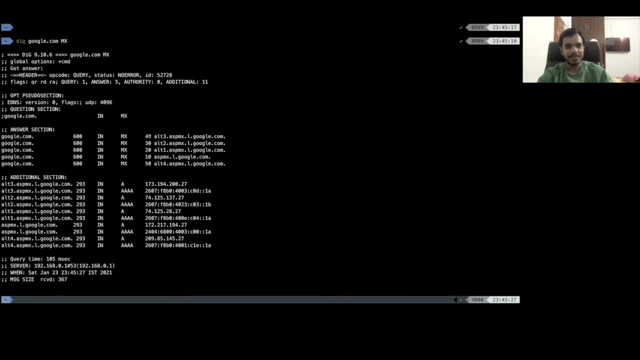 mx is the MX record, And then this, this one- I do not know what this one is- 40 and 30,, 20, these are all. So you can find out this and comment so that I also know this, And then you have the actual. if you see, these are the account and host name of the mail. 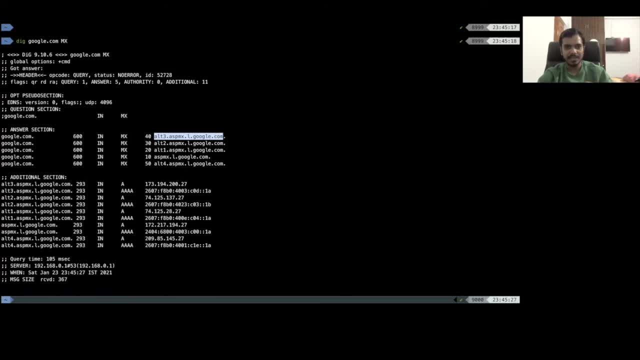 servers of googlecom. Again for additional section. you will see the IP address. like for all of this five host names that you have, like both IPv4 and IPv6 address, one A record and one in four A record. you can see it. Let's now come to the DNS message format. 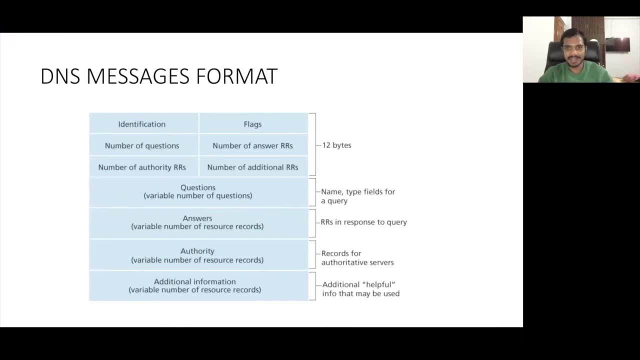 So we have already seen this message format in all those commands, but I'll explain that again. So see this first. so this is a DNS message format. This will be same for DNS query as well as DNS reply, Both for both of them this will be same And if you see first, 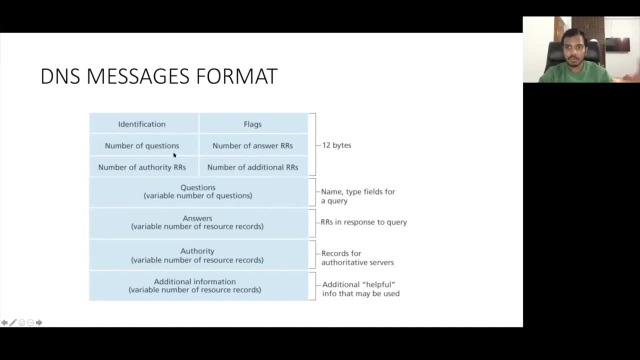 12 bytes. you have identification flags. how many number of questions are there? how many number of answers RRs are there? resource record are there. how many authority RRs are there? how many additional RRs are there? So this will be in the first 12 bytes. In the next you will have 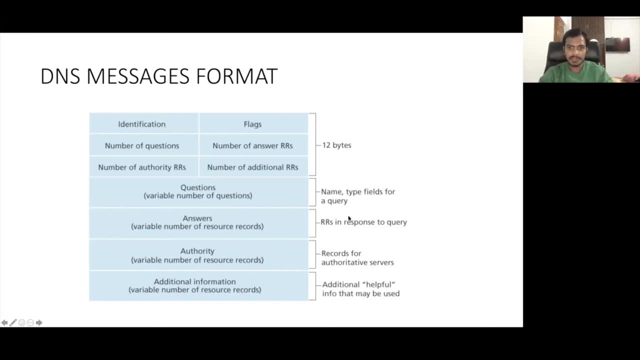 questions like what question you are asking the DNS server. Next will be RRs in response to the query. So these answers will see what I told you. This same as format will be followed for query as well as a reply. But again, you know that in the query questions will be there. 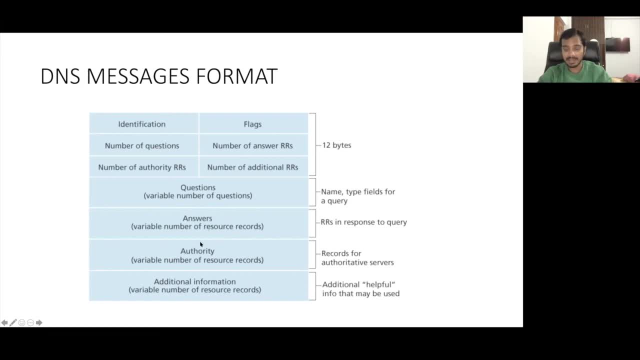 but in the reply answers will be there And in the answer in the reply also, authority will be there right In the questions. you will not have authority section. See this is answers RRs in response to a query. answer section. 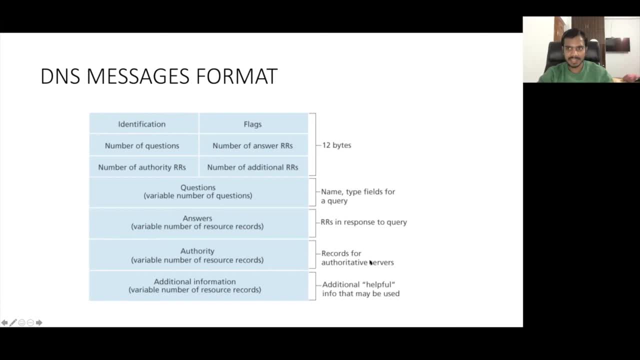 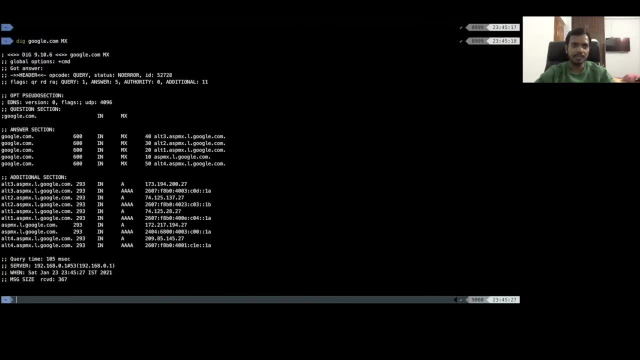 Authority is a record for authoritative servers, as we have seen when we were querying the root in a server and all. Then you have additional helpful information that may be used. So let me do one thing. I will show it here. They add the rate of this one right. 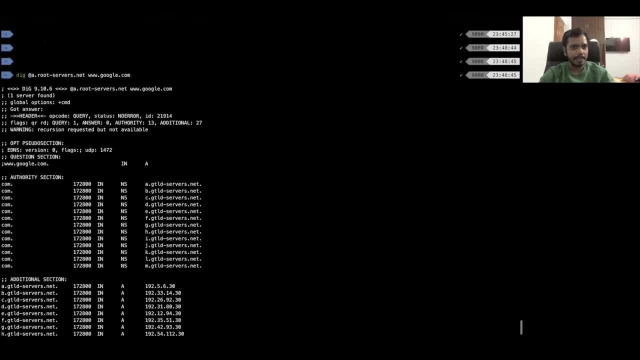 Root in a server we are hitting. You can see here like it starts from here. You can see flags are here. This is the type of query status: no error ID is there? some data is there? Number of queries: here is one. 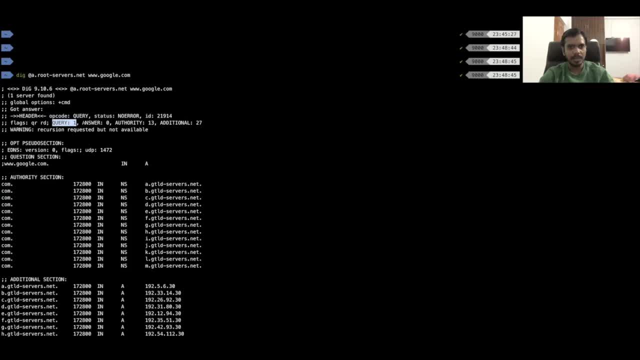 Like we are doing only one query, That is, what is the A record for wgooglecom? Answer is zero because root in a server does not store the answer for this. whatever question we are asking, But authority section, there are 13 resource records. 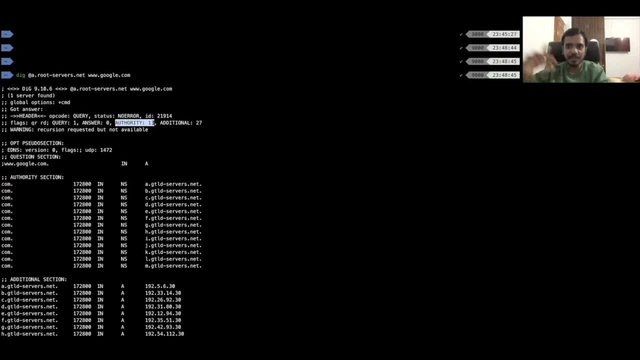 because this root in a server does know and it can point out to other TLD DNS server which can help us in finding the IP address of wgooglecom. Additional again, there are 27 kind of records here. So the question here is that for wgooglecom. 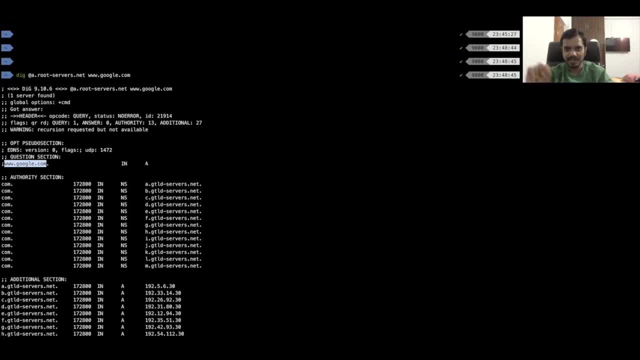 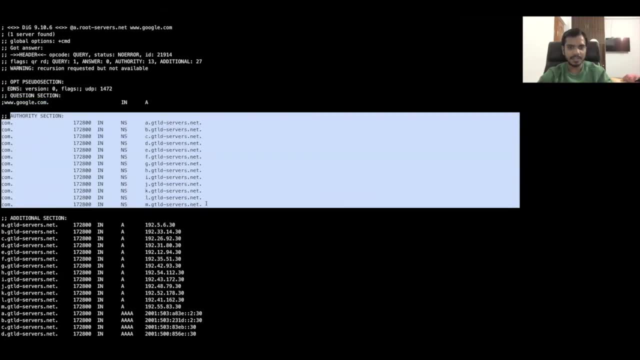 what is the A record Basically, what is the IP address for wgooglecom, So what is there in the A record of this? And then you can see here authority section is there. These are basically NS records which can help us in finding the A record for wgooglecom. 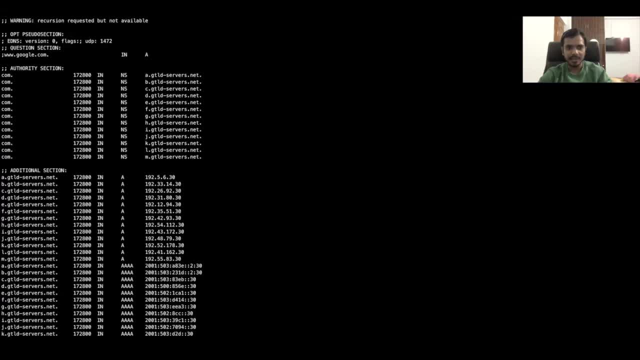 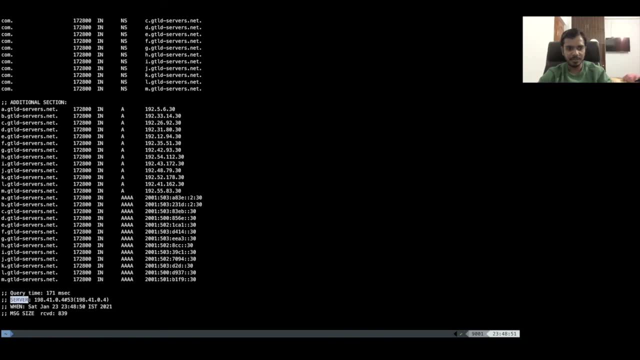 And then additional section, of course, you have the A records like IPv4 and IPv6 address And at last also you have how much time the query took, which server did it hit. So if you see, this is the IP address. which server did it hit? IP address of the root DNS server itself which we were hitting And port number 53 is there, Of course, for DNS port 53 used for communication. And what time this query? when we did this query? 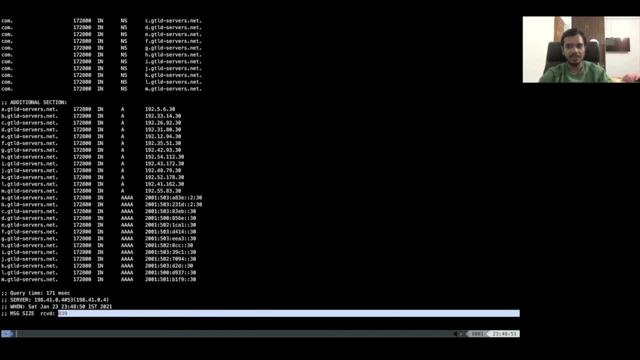 then what is the message size? received: 839 bytes. So all of information is there in the additional section. Now, of course, if we see, this answer section is not there because root does not contain the answer, But for that what you can do is if you hit. 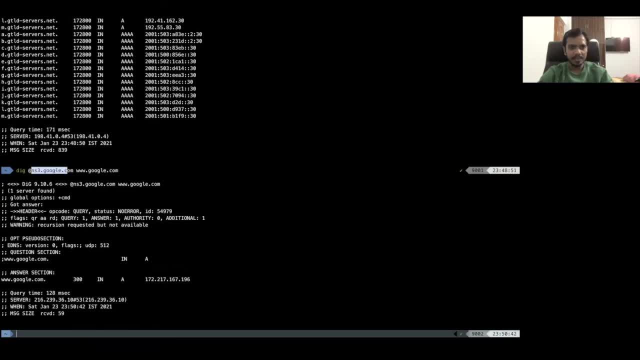 this one. basically, we are hitting one of the authoritative DNS servers And this will actually contain the answer for our question. Our question is: what is the A record for wgooglecom? And we know that Authoritative DNS server will show the answer. 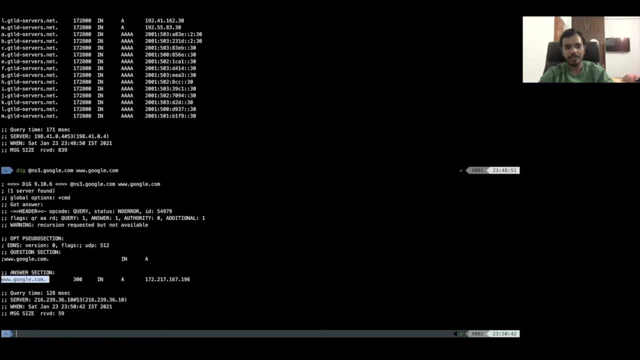 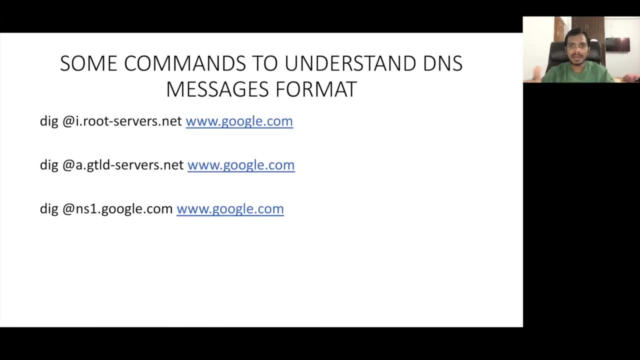 That's why if you see in the answer section you have wgooglecom and all of the A record and again the answer: what is the IP address That is there in here And here you have some commands to understand the DNS message format. 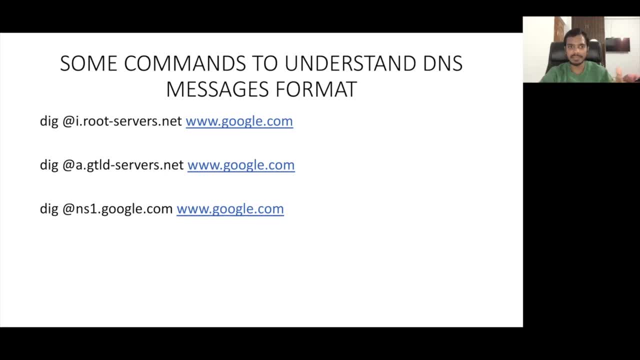 Like I have already shown you by running these commands: dig at the rate root server, Then dig at the rate one of the TLD DNS server. At last, dig at the rate one of the authoritative DNS server. 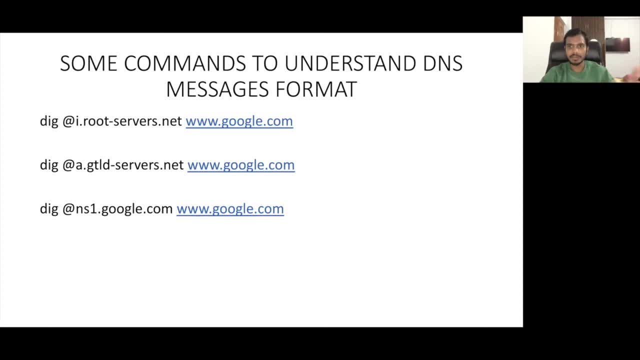 So you can also do this practice on your laptop itself, like on Mac, Linux and even using Docker also. Like Docker I have discussed in one of my previous videos. in the 10 late videos I have discussed about Docker, So that also you can use to run these commands. 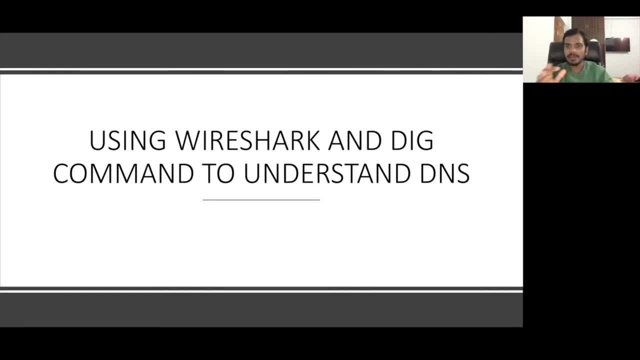 So that's all about this video on DNS message format, But we will again. one more video is remaining on DNS, that is, using wireshark and dig command to understand DNS. So of course, we have discussed dig here, But I will discuss about one important like dig plus trace, that is, the dig with trace. 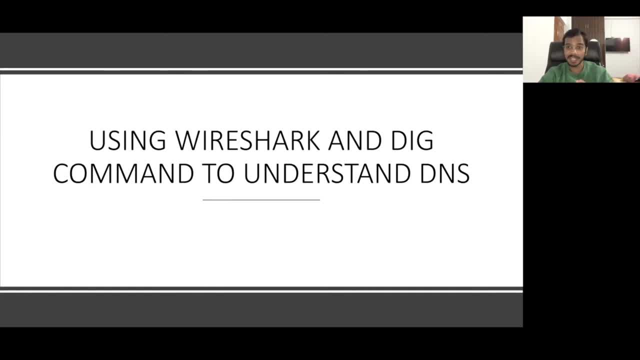 option. So that is very useful in debugging DNS And through that also you will understand how DNS actually works. And of course wireshark: I do it for most of the application layer protocol For HTTPS. I have done. 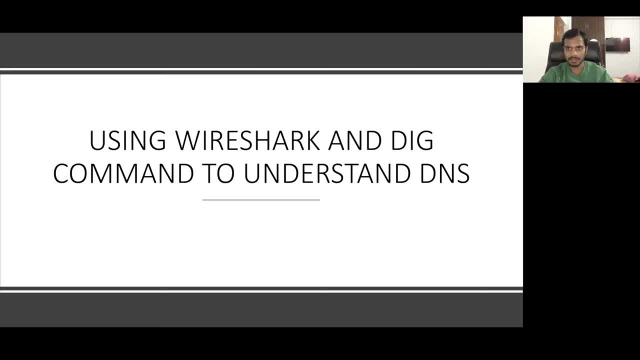 For HTTP I have done, And similarly I will do that for DNS also, Because through the wireshark you will be exactly see what is the query going from your like, from your network. So that's it, Like from your laptop to local DNS server. 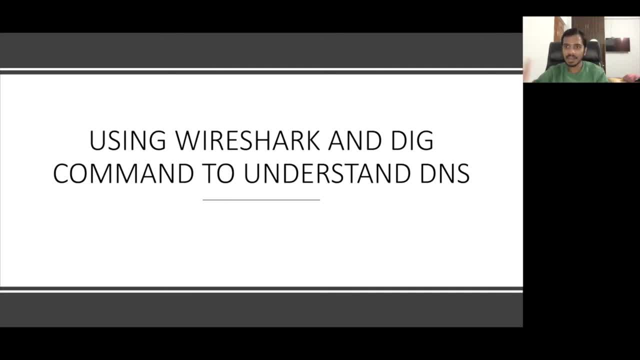 And we will also see what queries are going for local DNS servers. That also we will see And what exact reply we are getting in the wireshark. We will see all of that, All the fields that are there in like packets. So that's all for this video, Thank you.